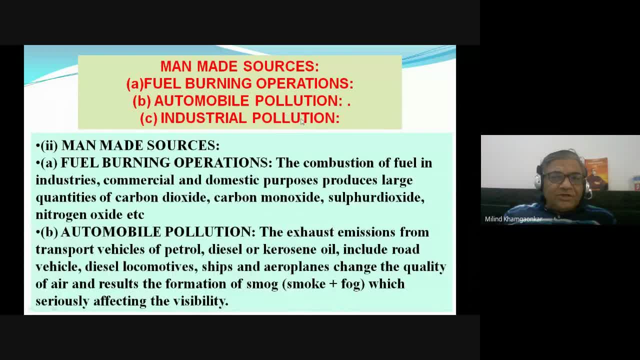 automobile pollution. and third is industrial pollution. The title in itself explains what is hidden there: Fuel burning operation. Either in our society, in our houses or maybe in certain social gatherings, etc. we burn a lot of the fuel. It may not be a wooden fuel, It may be a wooden. 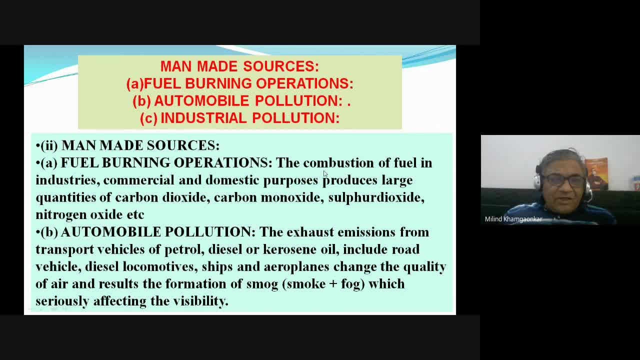 fuel may be a petrol, may be a diesel or any other type of the fuel, And as all this fuel contains carbon, So after combustion of this fuel, either in our house-to-house household purposes or industries, commercial or domestic purposes, produces large quantity of. 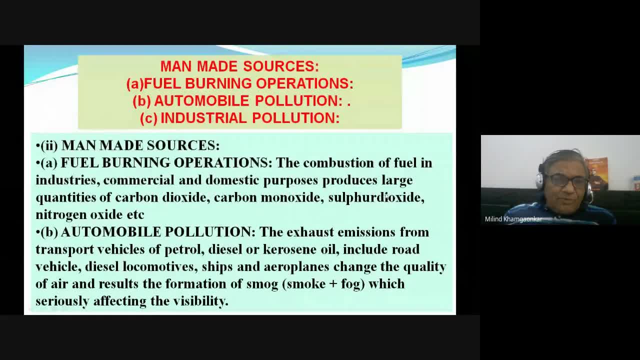 carbon dioxide, carbon monoxide, sulphur dioxide, nitrogen dioxide, etc. and this carbon dioxide is called as the greenhouse gas- Greenhouse, if effective, you must be noting. If we have, we'll have the time or the lecture, then we will definitely discuss about the greenhouse effect. it is part of our 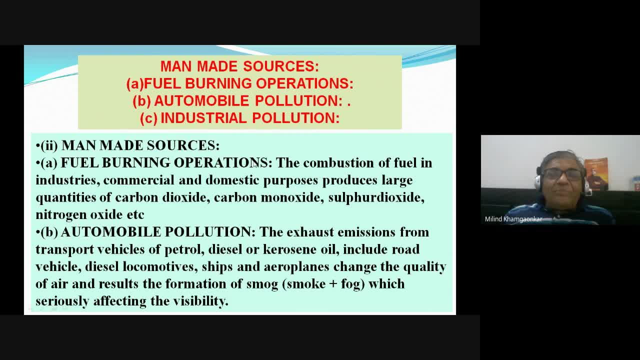 syllabus. so this fuel burning operation is one of the source of the pollution. automobile pollution, again. no need to explain various types of the automobiles: two wheelers are there, four wheelers are there. trucks are there. aeroplanes are there. railways are there. they run on the petrol, diesel or kerosene and during their running, during their working of 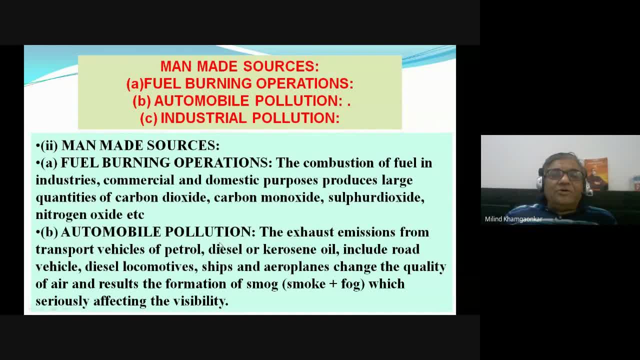 the engines. they produce lot of the carbon monoxide. in addition to carbon dioxide, they also form the smog, that is, smoke and the fog. smog means what smoke, and the fog, which also situations, obviously affects not only our lungs but visibility. so these are the dangers of the 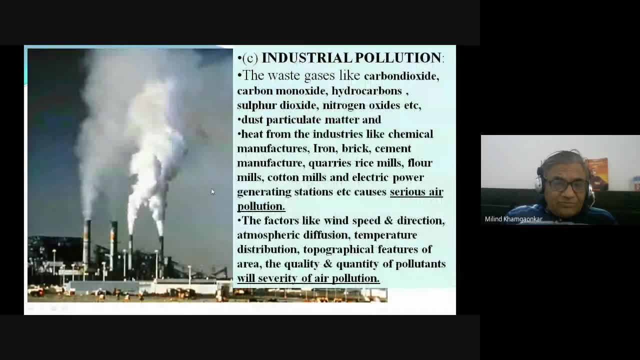 automobile pollution, industrial pollution. as you can see in the photograph, various industries. we have the cloth industry, we have the paper industry, we have the steel industry, we have the thermal power plants, and huge, because industrial development is going on all over the world. without industry we will not get the products. 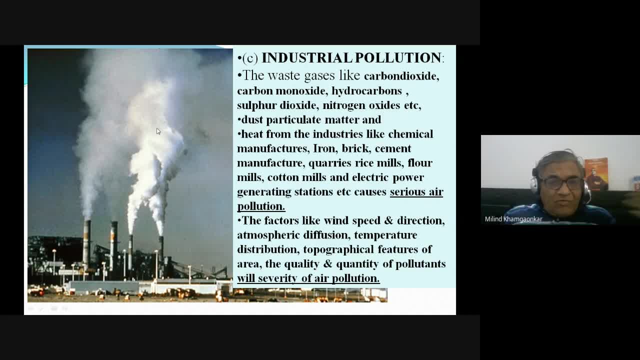 again. these industries are needed for our day-to-day livelihood, making comfortable. but these industries unfortunately produces the gases like the carbon dioxide, carbon monoxide, hydrocarbons, sulfur dioxide, nitrogen oxides, dust and the particulate matter. heat from industries like the chemical manufacturing, iron, brick, cement manufacture. 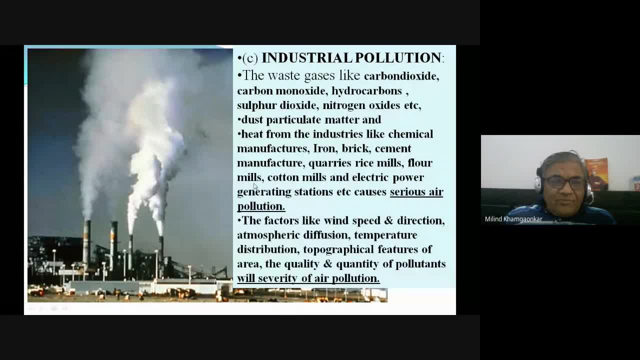 quarries, rice mills, floor mills, cotton mills, electric power generating stations, power plant, so all these industries causes serious air pollution. and though we provide this tax stacks or the chimneys, if you will take this elective air pollution in your final year, then you have some numericals on this tax deciding the heights of the tax tax. so therefore, for 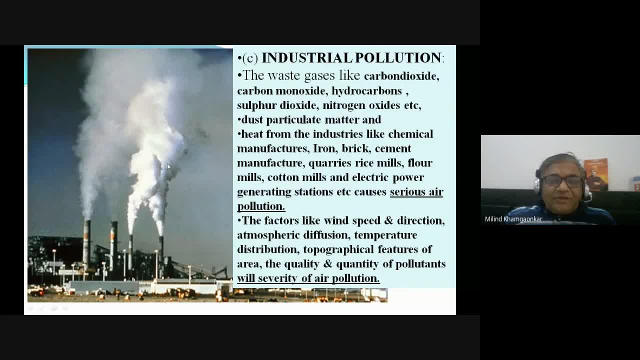 distribution of this smog, that is, the fog smoke and the mist, or the fog that is called as the smog. the factors like wind speed, direction, atmospheric diffusion, that is, mixing of all this smog, temperature, distribution, topographical features of the area, the quality and quantity. 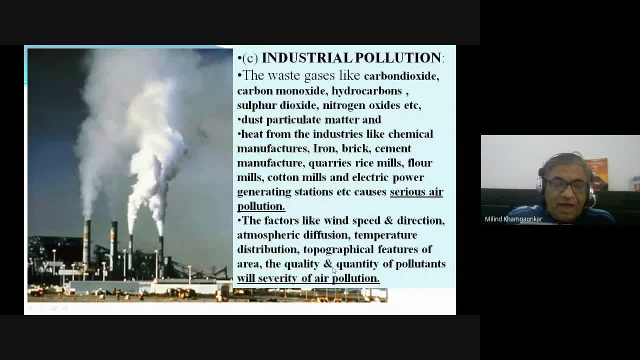 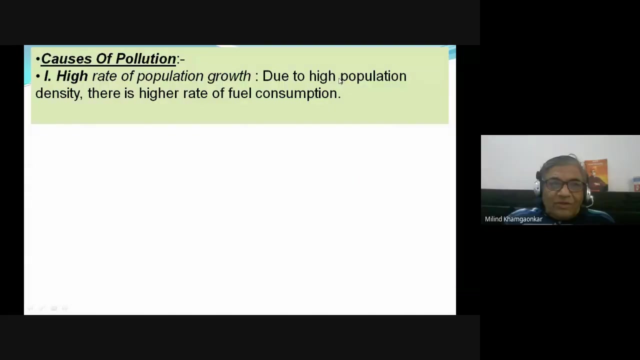 of pollutants will see, will have the severity of air pollution, visual me and quality of the pollutants. so all this affects the air pollution. now the other causes of the pollution, other means, the sources we have seen now the various causes of the pollution: the high rate of population growth due to high 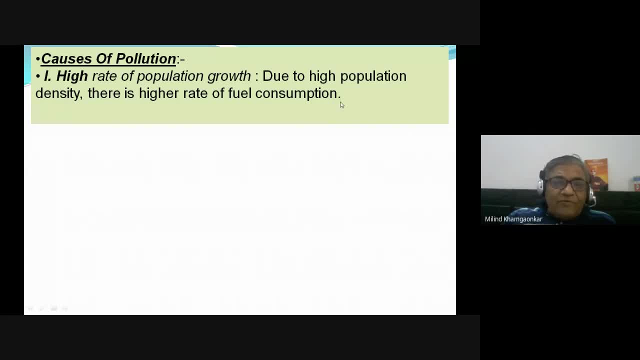 population density, there is a higher rate of fuel consumption, energy, the amount of people is increasing. due to that population growth, all the necessities has increased. So this population is one of the cause for the pollution. so high rate of population growth is one of the cause only in world. 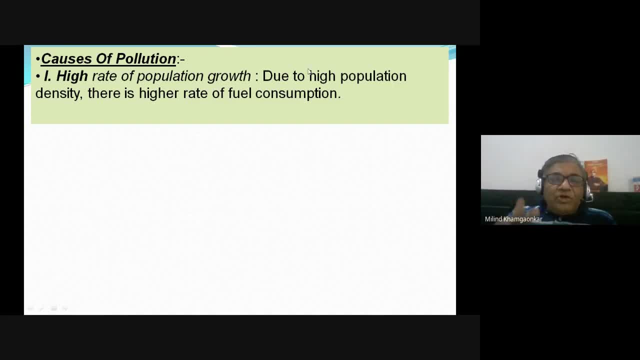 There exist only two countries. the population is much higher for India & China as compared to India. China at least 30% of the population, has high population diversity, have more topographical area as compared to india, but but india is having tremendous population. therefore we are facing all these problems. 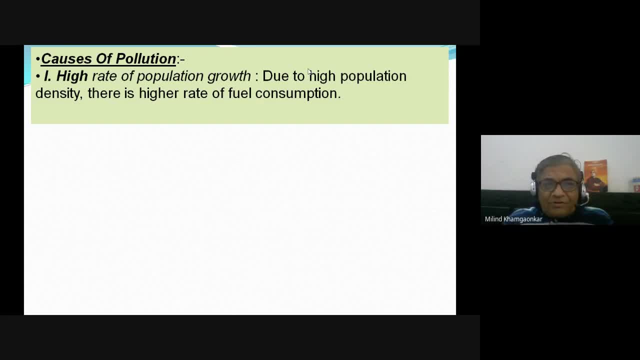 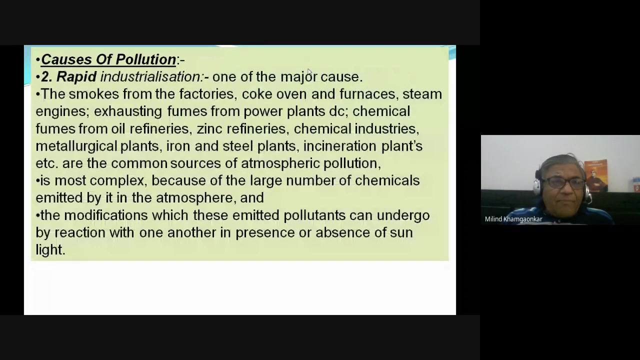 in addition to pollution, employment problem. so we must have something to control this. rapid industrialization is another cause of the pollution again, as the population is, more the need, the requirements are more the kapra jada lakta khana, jada lakta hai motorcycle, hai mobile sabko, lakta hai roads hai sabko. 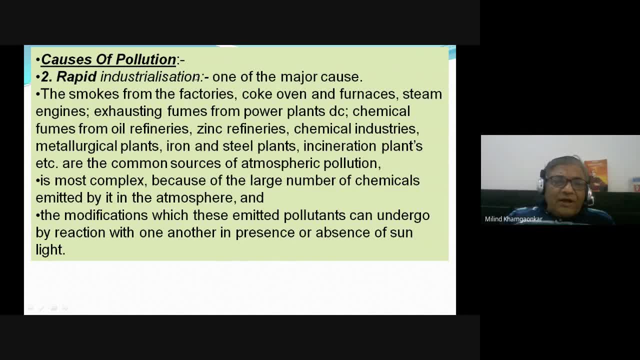 hai ghar lakta hai, chappar hai to uske karan. industry bohot bad rahi hai. one of the major cause: the smokes from the factories: coke, oven and furnaces, steam engines. some fumes exhausting from the power plant, renting from the seal plant, chemical fumes from the oil refinery, zinc refinery, chemical. 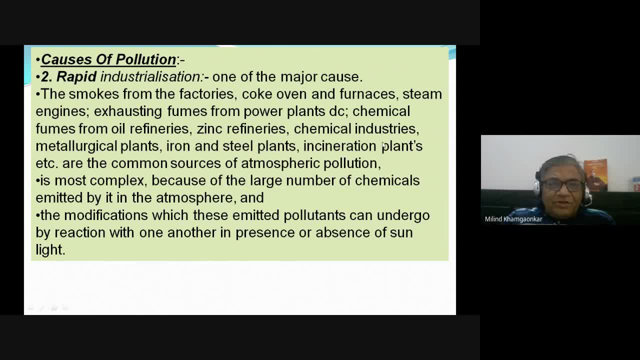 industries- metallurgical plants, iron and sea steel plants, incineration and a gelane valley plants are the common sources of atmospheric pollution and they are very complex because of the large number of chemicals emitted by them in the atmosphere. the modifications which pollutants can undergo by reaction with other, in presence or absence of sunlight. 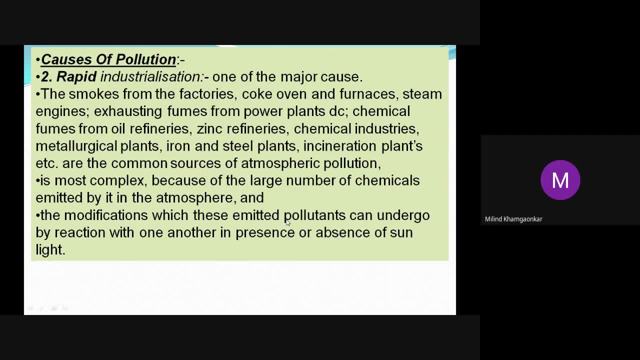 is again more complication and I'll be on primary or secondary of the pariah Polly, types of the pollutants: primary pollutant and the secondary polluted. so yeah, Joe, Allah, Allah, industry sip pollutant nickel today, a kadeh zinc factories, a kucho or chemical nickel Tyre oil refinery, say Joe. 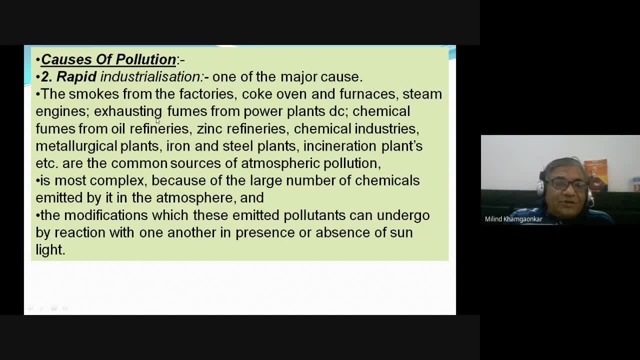 Mathura oil refinery. a US message. sulfuric acid SO2, nickel, Tyre, SO2, SO3- unstable SO3, it be it mixes with the water or the water vapor in the atmosphere, converts to H2SO4 and then again spoils not only buildings, which 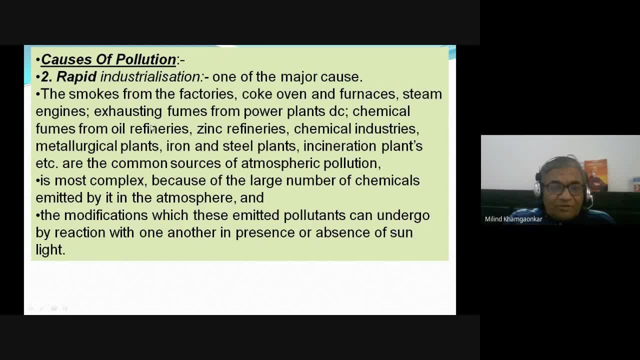 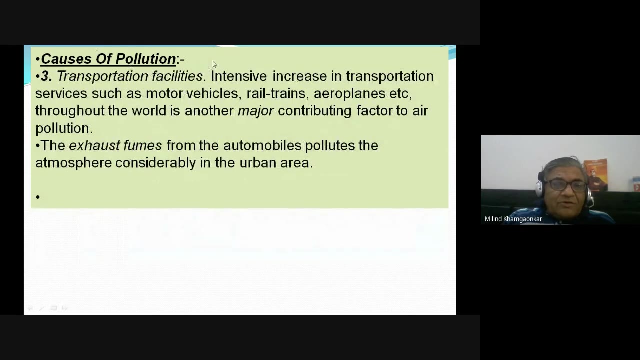 are coming into their path, but also affects to the human beings and the animals also. so therefore the primary pollutants affects and the two pollutants together also affects to the all these human and the animal race, etc. so the that is one of the cause of the industry, that is the 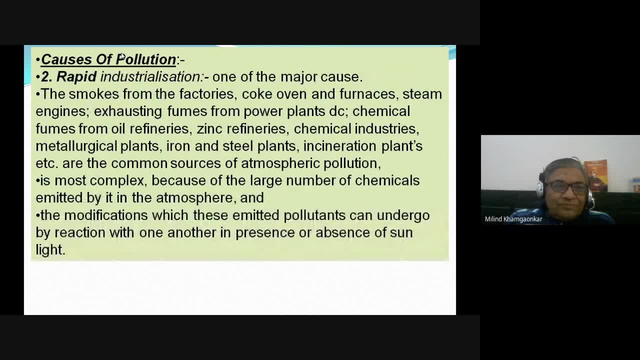 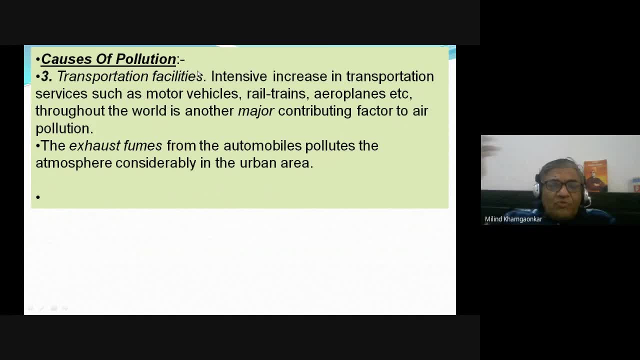 industrialization, rapid industrialization, you know, which lead us here be Salma coffee, fast industries, but the motorcycle, agree, here I got a motorcycle key factory to nine. a motor in my days- in my days means in 1980s- there were only two, three scooters. 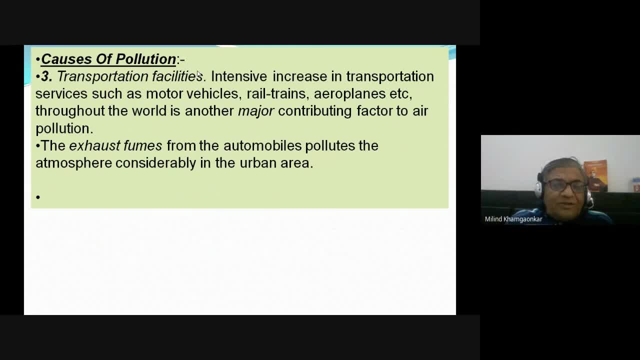 were there by that scooter. we is there and the Lamberta was the old scooter was there. now the various types of the scooters and scooters are their motorcycle. only the Sawa motorcycle was there and the rajdut motorcycle and the bullet was there and it is very difficult to get the bullet. now numerous motorcycles, Honda. 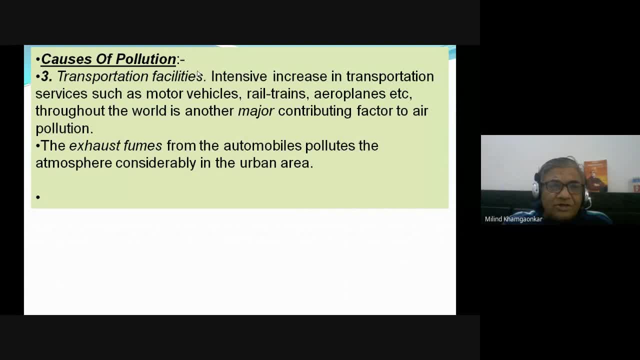 honda and whatnot, Yamaha, etc. so the industrialization has definitely polluted our atmosphere, not only atmosphere but water and all the things. transportation facilities again, vehicular transfer, vehicular facilities intensive. my wish we can manage more aquesta ik coupe e дело, start big router. 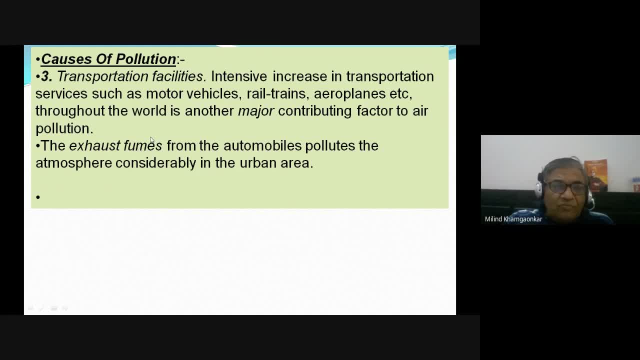 go, come past gym. goal a, b, b, g, e. another car ad tomorrow. ha pollutes the atmosphere considerably in urban area Amarjo shahri, bhagia, who's map ko bahut, bahut garmi miliki. auto, automobile k, karan vehicles k. 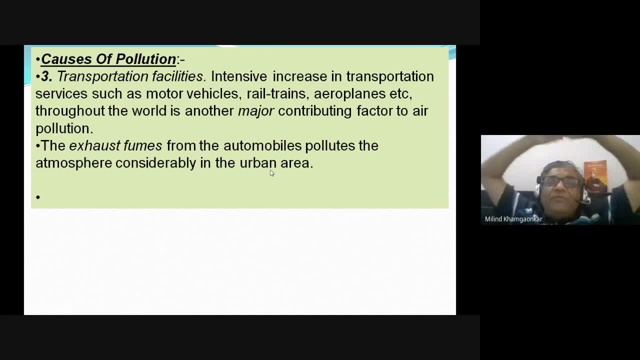 karan, if you are living in Nakpur and if sometimes you get the chance of travel in the evening from Gandiva to say some shivaji nagar or the survey Nagar, trimurti nagar, etc. so if you start from Gandiva you will notice there that in 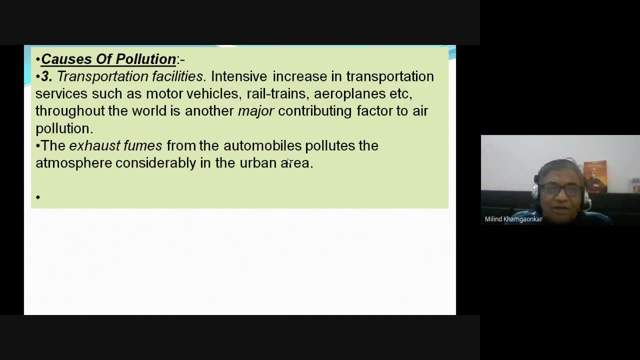 the evening, the Abito corona heto breakdown, a naked job or a full swing. may traffic rate is up to wood, or both. apnea apk jalan o t has met a clue. or Jesse a pashyam nakur kitar of at a. as soon as you cross the birdie, you will feel. 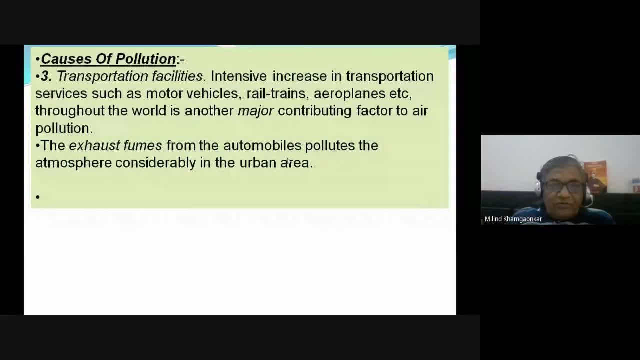 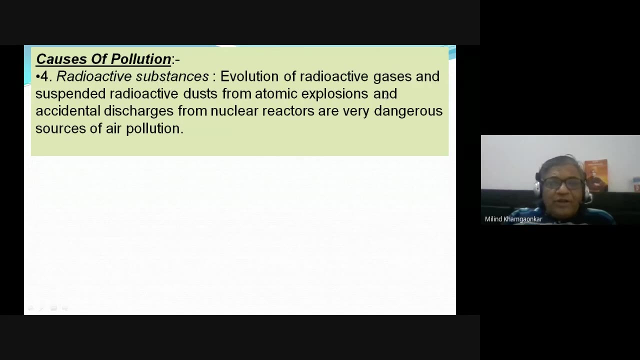 very pleasant and nice weather change. so that is all due to the transportation facilities, the automobiles, which pollutes the atmosphere, and there there are certain radioactive pollution, also there, due to the radioactive gases and suspended dust from either atomic explosion or accidental discharge. you, for the nuclear reactors are very dangerous source of air pollution. 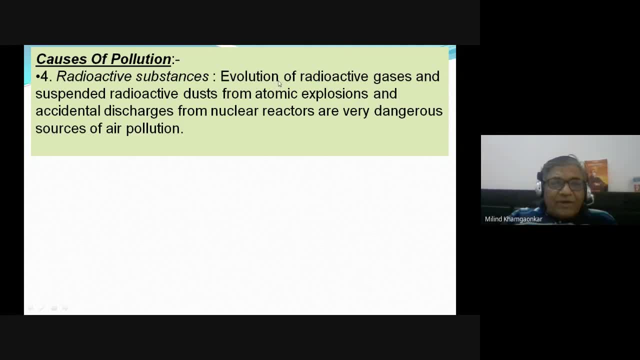 thinking I said Chernobyl may have a doctor, Russia may you have the atomic energy plant, jojo. hey, where do we lose? mainly cages over explosion, or go to this offer over a and that has created lot of the cancers. chair, no, bill up net pedicure there. the radioactive substances, k, karon, hosta, and therefore there is a lot of the cancers Chernobyl you can see on the net. 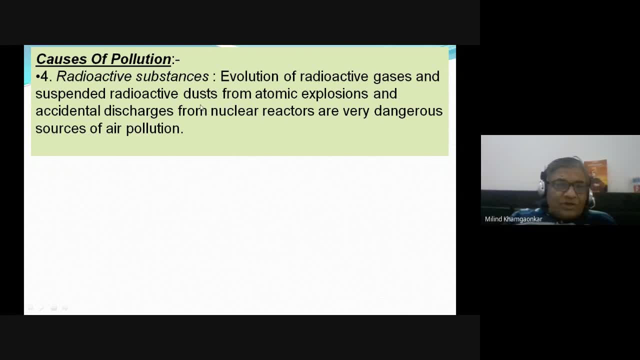 that you can see, by the radioactive substances today, when they have reactivated this nuclear power plant substances now it may be very dangerous, but that is hard to say. but but this is what we are doing because the nuclear reactors are, levels are very dangerous. so, although people are also, people are very dangerous. so the nuclear reactors are very dangerous. 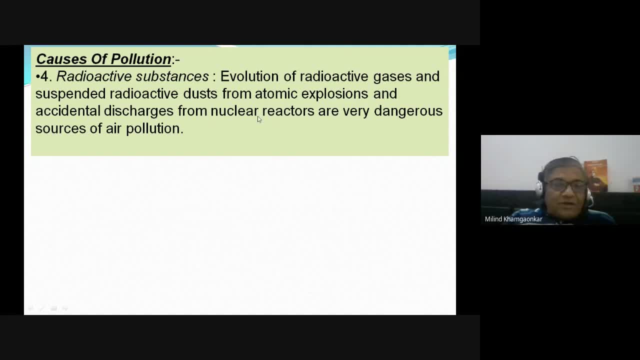 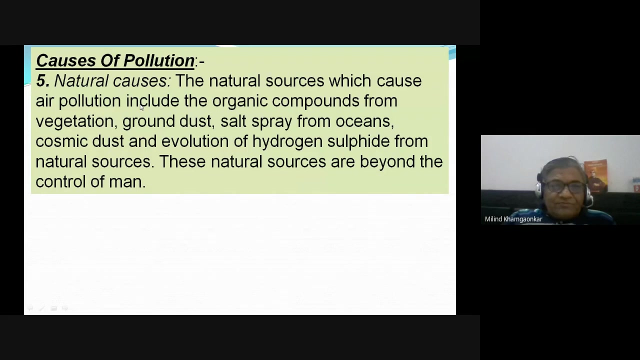 radioactive power plants are there? atomic power plants? they give the electricity in a very lesser cost, but the danger of radioactive explosion is there. so these are the four important causes of the pollution, certain. now, these are all the man-made causes. now the natural causes, nicer geek Rita. 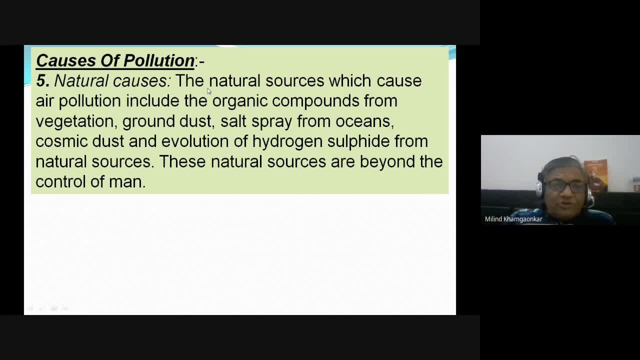 Keisha. what are the natural sources which cause air pollution, including organic compounds? decomposition of organic compounds from the vegetation, ground dust, salt spray from oceans, cosmic dust, evolution of hydrogen sulfide, of sulfide from natural sources. these are the natural sources which are beyond the control of the man. okay, so this? 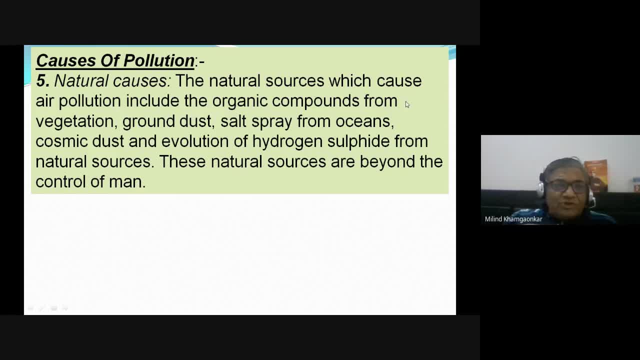 are the natural sources, that is, the decomposition of organic compounds from the vegetation. your tool would be a jamin kew per se. how a k current, yeah, deserts out there. that is the ground, dust which also spreads into the atmosphere, some salt which is emitted from the oceans, or the seeds, because the 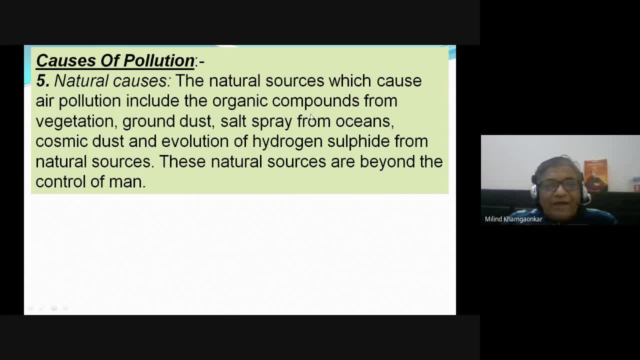 sea water contains the salt. due to the extreme heat, the salt gets sprayed into atmosphere. the cosmic dust, you know, Joe, Joe and Terrell say your dust at the air. wait whom? Ketu yata, hi, yaka ya? or, which is a enthral me with the head of us. 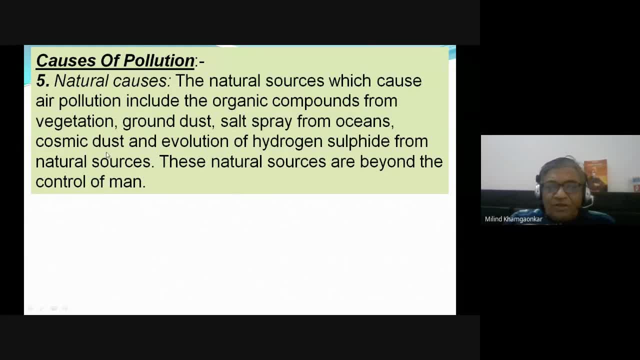 cosmic dust, curcumin, the woe be that also is the one of the cause of the pollution: air pollution, hydrogen sulfide, evolution from the decomposition, etc. from the natural sources. so these are again. the volcanic stuff is there or the volcanic gases are there, desert. these are all. the. the winds in the desert are the natural causes of. 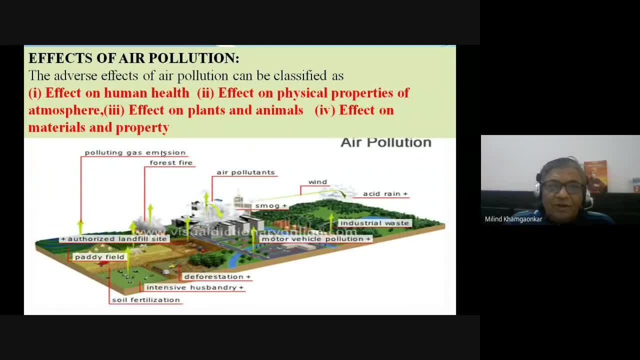 the pollution. now we will move on to very important part, that is, the effects of air pollution. though we know all these things, you know air pollution koi hamar liye naya hai, kya bilkul nahi hai. on the contrary, we we may be knowing more than this, but we are. 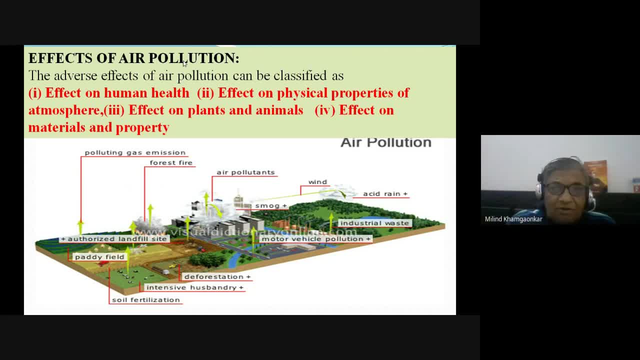 fitting them as per our technical requirement and as per our syllabus. so now we will be moving on to the next part of our discussion is the effects of air pollution. the adverse effect of air pollution can be classified as effect on human health, effect on physical properties of atmosphere, effect on plants and animals. 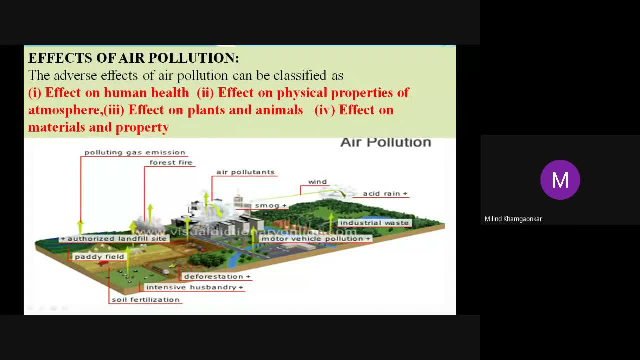 and effect on materials and properties. again, a self-explanatory photograph is there. you can see the air pollutant there from the industry. the smog is there also. enough again, the combination of the fog and the fume that is the smog, or smoke, smoke and 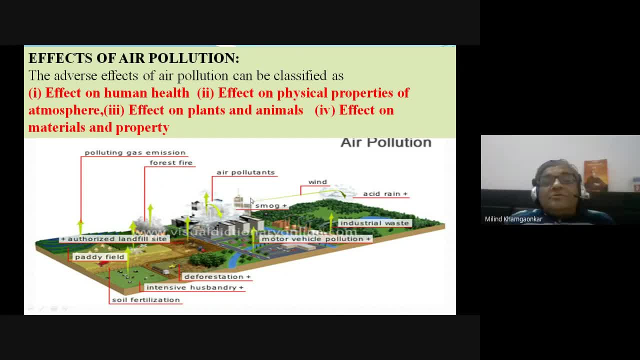 the smoke. along with the this thing, water vapor, is called as the smog. so smog is there. wind helps to spread all this air position as a result of the air pollution as well, so as we can say, as if this air vivir is placed on the air in an environment where 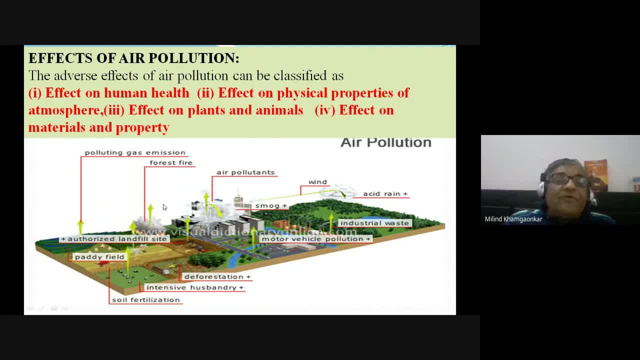 there is an air pollution and air pollution. there should not be any air pollution there, pollutant. it affects the forest, it affects the agriculture, paddy crops again. motor vehicle: motor vehicle pollution is there. industrial waste pollution is there due to this smog mix with water or the rains causes the acid. 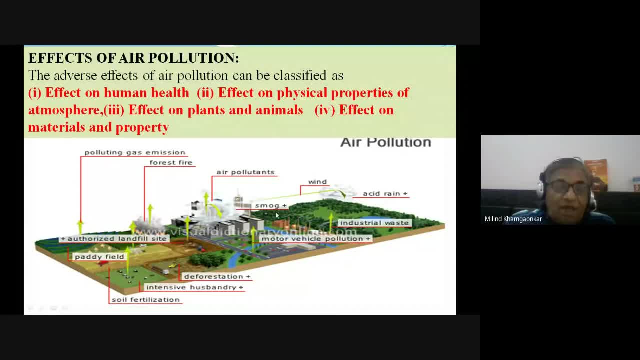 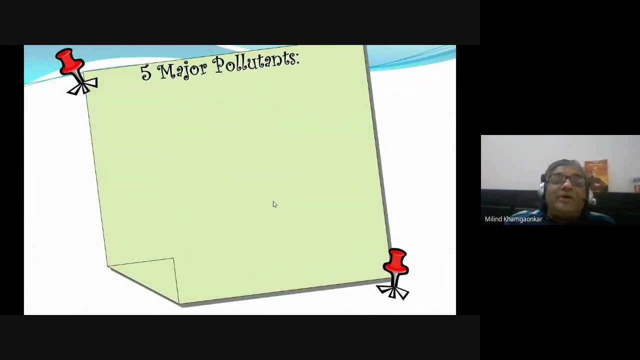 rain also. so how this affects to the surrounding of the sources of pollution can be seen here also. humans are affected. how they are affected, that we will see in the our next slides to come. these are the various polluting gases. you can see major pollutants. they are the carbon monoxide. they are the 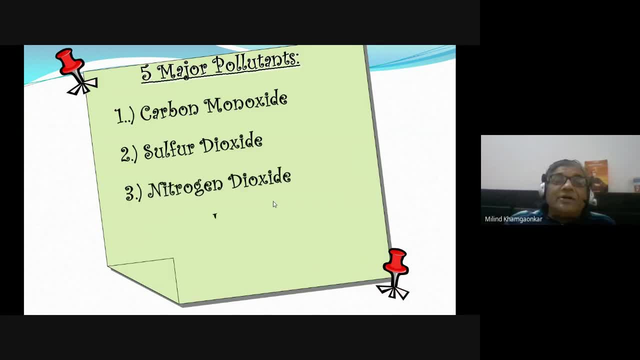 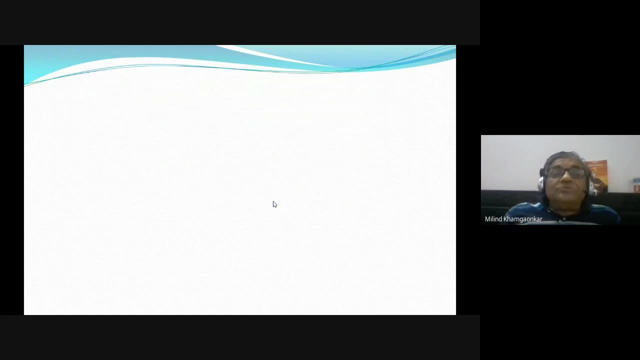 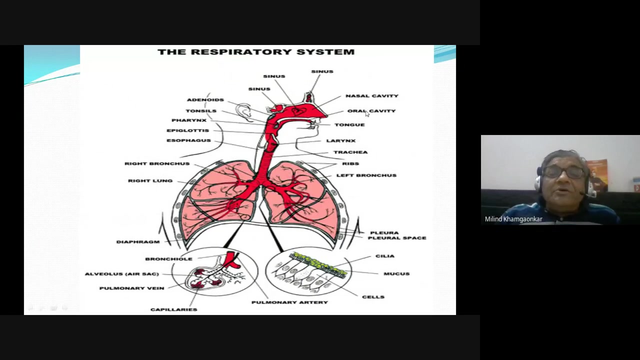 substances that are produced by the produce. we know these are the substances: sulfur dioxide, they are the nitrogen dioxide, they are the particulate matter: Barik, Jupiter particles, ready or ground level ozone. all these five contribute to major pollutants. you can see how they affect to our respiratory system. this is 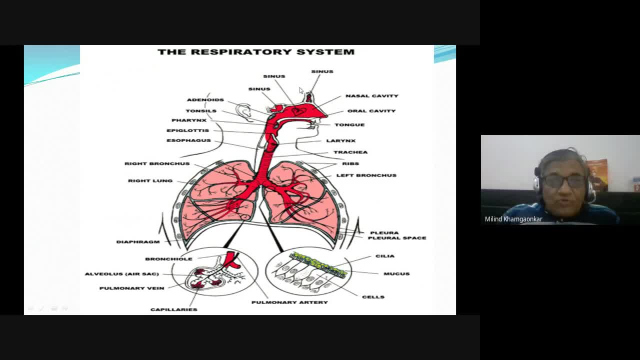 all the respiratory. a discourse wasn't sounds- table to him in the way the vahasa JSA. through this nasal cavity, all this pollution enters and spoils our lungs and the bronchies, etc. and I'll be Corona, be weak or I am are a lot came. 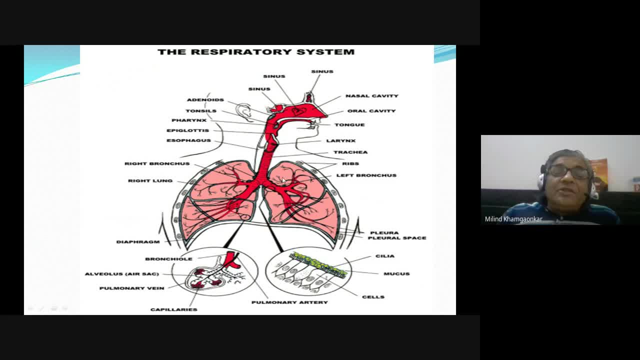 at them say I thought I was go proper treatment. maybe the world lungs cook haraap karta or fear Amari. oxygen requirement- yeah, oxygen inhaling, jo bowling a who come with a Jackie. hey, the quantity of oxygen in our blood reduces and then we start getting the problem- the same thing. 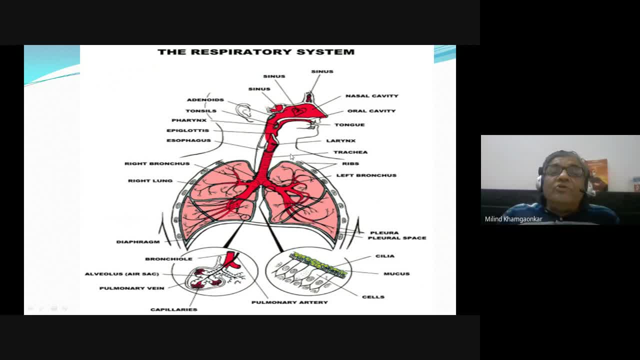 happens with this air pollution? okay, the smoke, the fog, that is the smog, etc. the, the fumes, the particulate matter, both, both jo, bari, bari, particles ready to occur, say, lady, to clear any of those if they are inhibited and uh, like the flash, etc. and 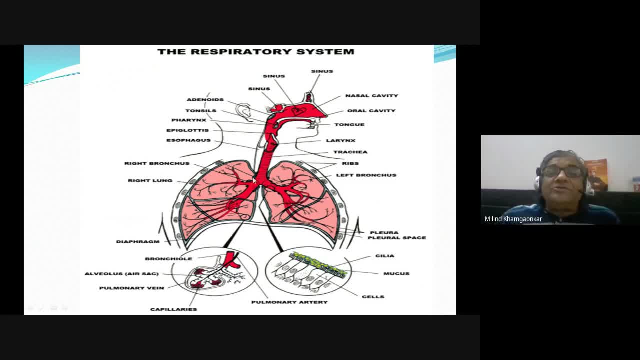 that will the most affected of varieties, that love, which is the second heart of our body, because these lungs supplies the oxygen for the burning of carbohydrates in our body. so therefore, the importance of the oxygen and the pollution. take now the effect on the human health, of the human health and the 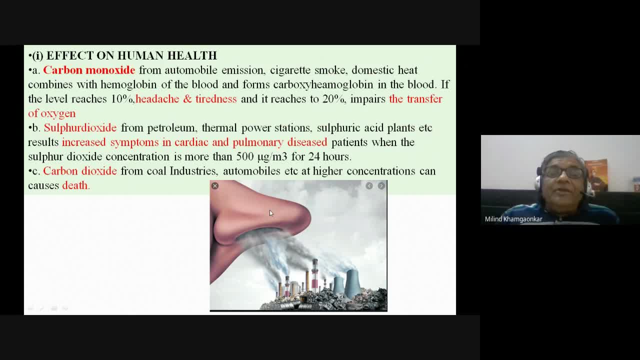 Again. I have shown you on your screen A nose is there, the photograph of the nose- And through this nose we are inhaling a lot of the pollution, Carbon monoxide, So both these things get deposited into the lungs. 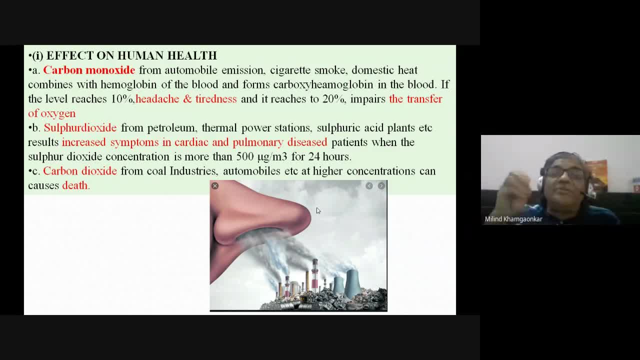 Carbon deposits. After many years of smoking the lungs get completely damaged. So this is only the cigarette smoking pollution. The other pollution is atmospheric pollution, the automobile pollution, industrial pollution. All this pollution affects our health. So the effect on human health. 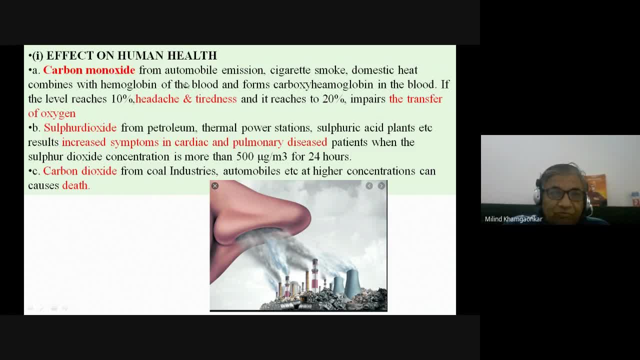 By the various gases that we will see. As I have told you, a short note is asked a number of times. Maybe in MCQ you may be asked: what is the effect of carbon monoxide, sulfur dioxide, carbon dioxide, et cetera? 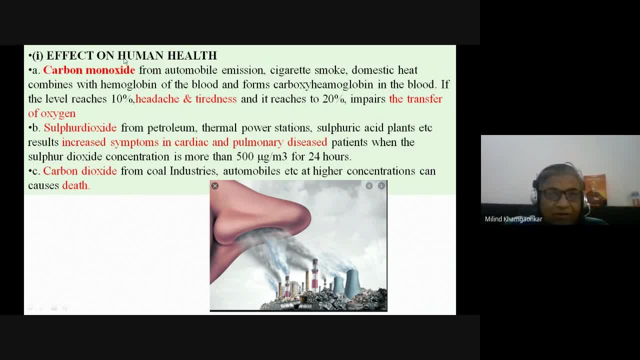 We'll see, one by one, Carbon monoxide From the automobile. we will see where from it is the source: Carbon monoxide, Automobile Emission, Cigarette smoke, Domestic heat combines with the hemoglobin of the blood. 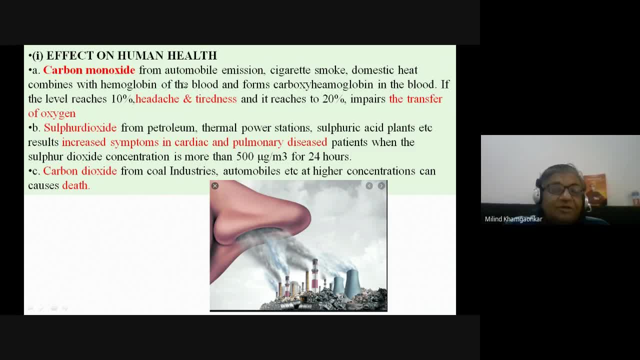 This carbon dioxide, carbon monoxide, this hemoglobin in our blood, this red color iron of the blood and forms carboxyhemoglobin in the blood If this carboxyhemoglobin level reaches more than 10%- 10%. 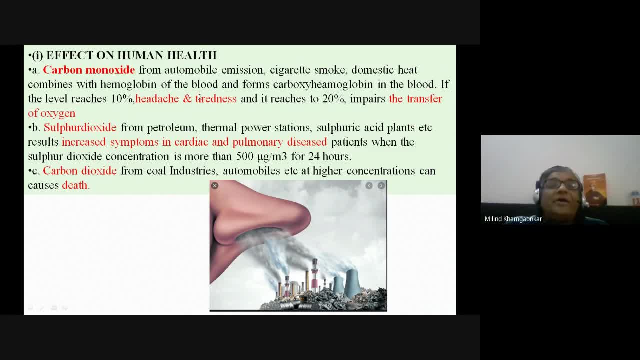 more than 10%, then hair headache and we feel tired. And when it reaches more than 20%, it affects the transfer of oxygen, That is, we begin to feel tired and the oxygen component in our blood begins to decrease. 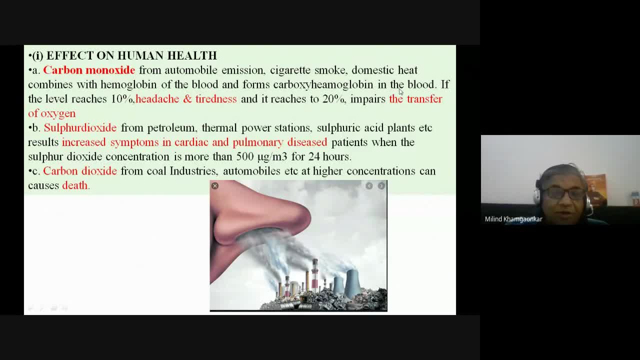 So this is the effect of carbon monoxide. We don't know whether it actually helps us. it is more beneficial, but the result is the result of tossing water, sleep, breath, And if it does, then it is automatically negative for us. 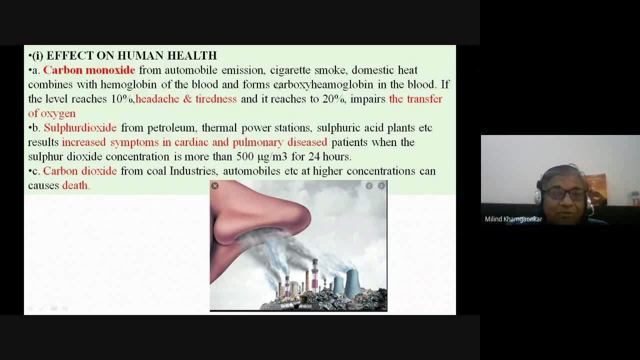 In fact it's the same thing. Yes, it is the other your expression on oxygen level sensitivity. It absolutely helps you. It also helps us, like with water crash. It also helps with BRA sausage. It's equal to that. 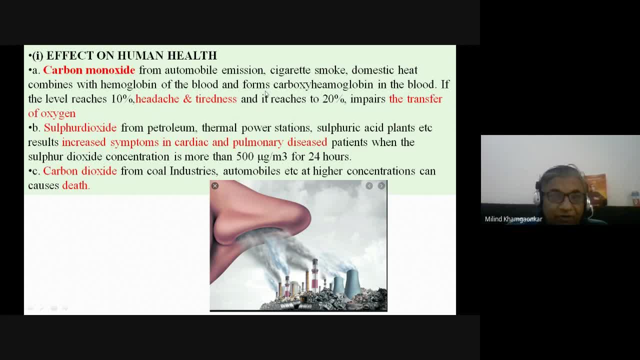 Is that right? Yes, Yes, It is Yes. indicator oximeter. so the carbon monoxide affects that oxygen in our body and that is the ultimate starts: failure of the lungs. so carbon monoxide, then the sulfur dioxide, so2. as I have told you, it is produced from the refinery, that is. 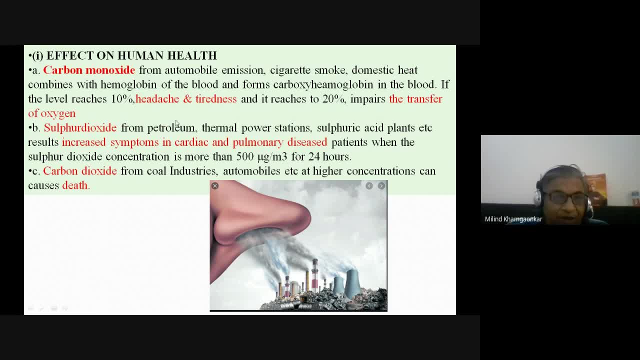 the petroleum refinery and up you have a from the petroleum liquid that is being brought from the my mines or from the petroleum factories it is being refined there in the refinery. the wahhabi, a sulfur dioxide, went. that thermal power plant me went. I am RS about you, but you may thermal power plant a karate thermal. 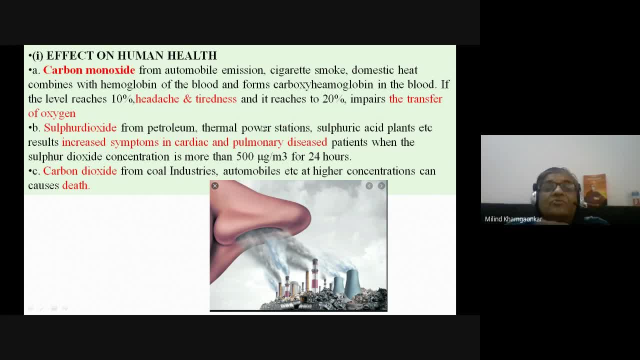 power plant. copper cannot. thermal power plant. you either general for the super thermal power plant- well, I am our apartment- or maria thermal power plant that produces sulfur dioxide. sulfuric acid plant, a khadaa, a sulfuric acid banana. what does? it is sulfur dioxide in the atmosphere. 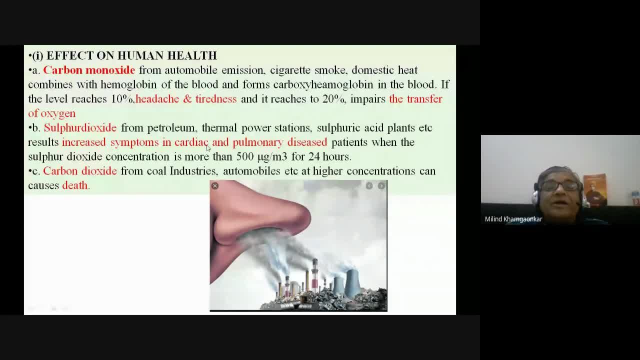 does. it increases the symptoms in cardiac and pulmonary diseases and a cardiac and a heart or lung disease. but I thought: yeah, Joe is ke baju me job e low reite hoon ko jada chances patients when the sulfur dioxide concentration is more than 500 micron gram in a micron, so micron gram in a gram divided by thousand. 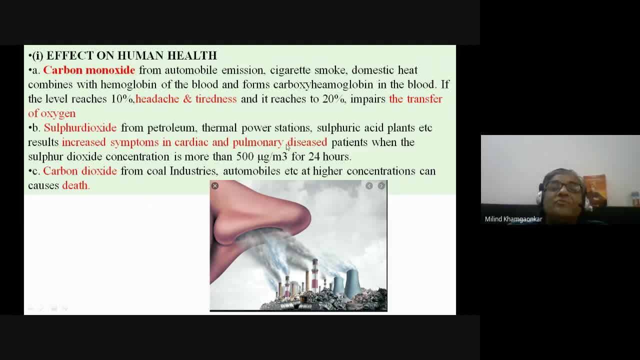 per meter cube for twenty four hours. per meter cube of the air, may 500 in 0.5 gram, you can say so, 500 gram, point 0.5 gram. yet even it, not but the hat. oh yeah, mariko, heart problem or lungs problem? karta, hey, carbon dioxide, co2 from the 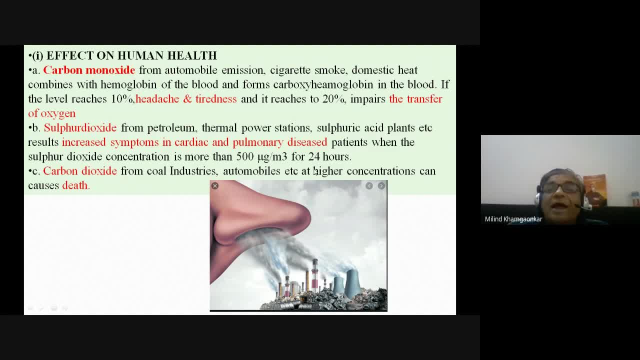 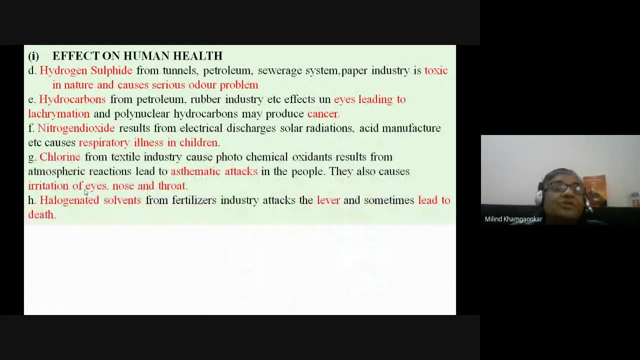 coal industry. automobiles at higher concentration can cause death. jada, carbon dioxide, Raha or a mariko inhale. oh yeah, Marissa Asus was a guy. oh yeah, Mari to kakarana was a tie. hydrogen sulfide, h2s from the tunnels, petroleum sewerage system. paper industry is toxic in. 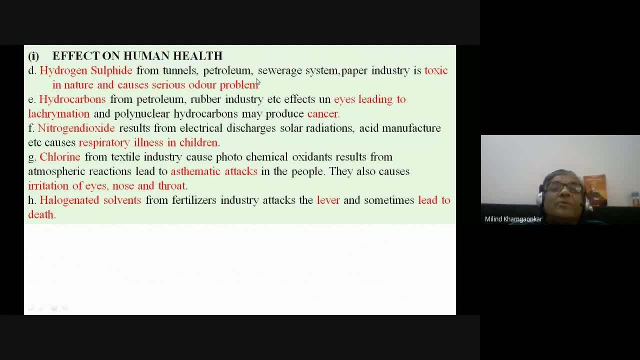 nature and causes serious odor problems. chicken is to ask a problem. is a camera boss sass lena kubi takla Karega. boss lena kubi takla Karega. or heart kobe baki bill lungs ko problem? create hydrocarbons from the petroleum rubber industry effects on our eye. a coco? 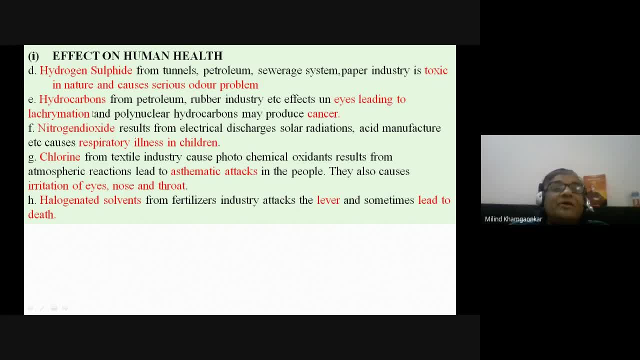 taklip data leading to lacrimation. and Pauline Pauline, nuclear hydrocarbons may produce cancer. so yeah, a coco hydrocarbons, oh hey, yeah may. a coquette readiness, disco, bullying, a general hydrocarbons are like a automobile industry, automobily, motorcycle, a petroleum, a it's. 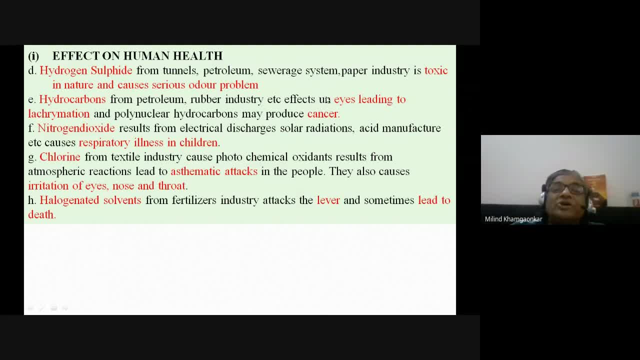 about sorrow the way they are. Maria Kameka, I took a general here, so that is the accretion. and if I'm both Java exposed, okay, y salota, Kena occupational has art car came ready. Katamara, I'm as Amara chavi is. I am her work, hydrocarbon. 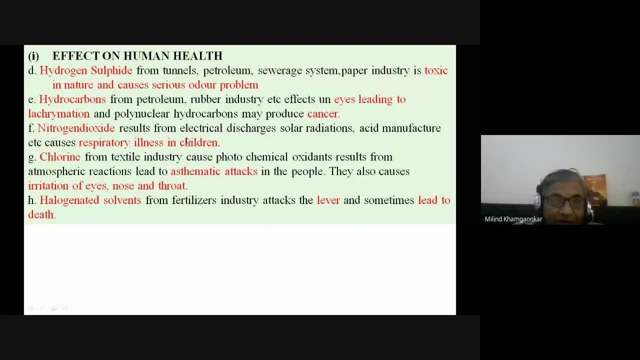 co-exposed Hotel. so a coca cancer? oh, subscribe nitrogen. nitrogen dioxide, a no to results from electrical decay charges, solar radiation, acid manufacture in a electrical discharges and a Joe welding over a cartel to us. may spark with a head to us. may nitrogen dioxide, Nikolai, who are my respiratory? yeah, they lungs. 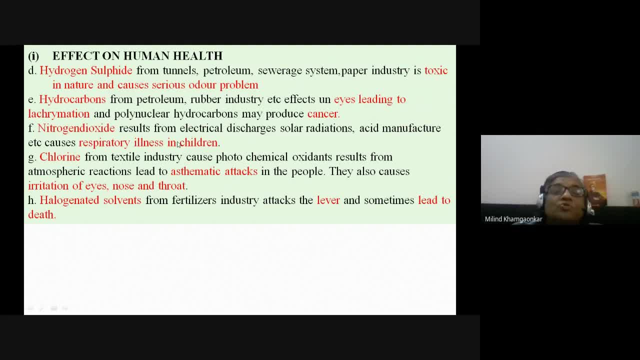 were garrick. a joy in the illness, a war, but choco, be the cleavage that I aqua cotta data here: chlorine from textile industry. chlorine, Joe, hey, from textile industry. cause: photochemical oxidant results from the atmospheric reaction lead to asthmatic. the matter casa in the people. they are also cause. 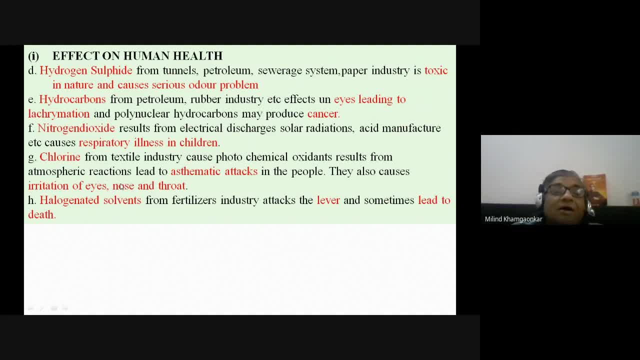 irritation of eyes, aqua key Jalan knock or throat, so ENT bullying, yeah he eyes, nose or throat ko Jalan Dega. chlorine atmosphere may both Jada Hato chlorine Jase he Bucky Joe a. halogenated, yeah, halogen solvents, Joe a. 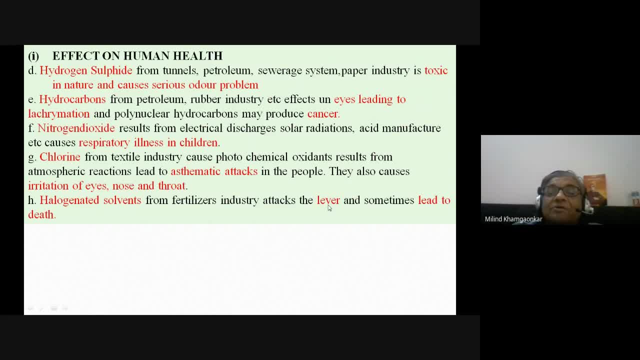 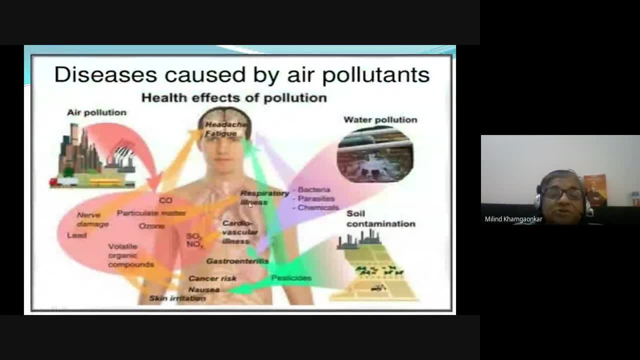 from fertilizer industry attacks the leaver and lead to death, again with the help of one of the sketch how the air pollutant affects various parts of our body. it a Kota hater, fatigue, brain may attacked, carbon monoxide, k current paki with an arrows, a particulate matter, ozone, etc. which part of the body gets affected is being shown here. one part of the body is affected is being shown here. one part is heart attack is caused by carbon dioxide and therefore the Portland effect is also due to the skin, by the pain, by the smell, by the smell of the skin and so many other things. 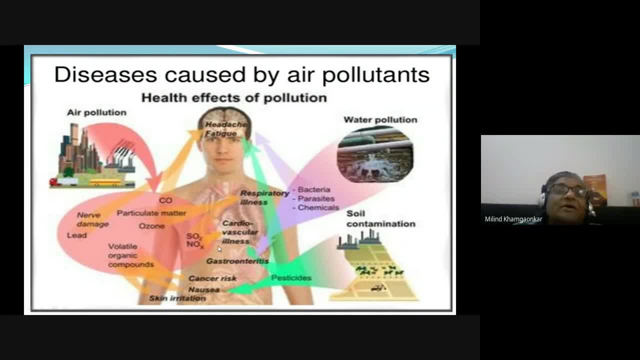 If there is water pollution, then our stomach will be damaged. What will happen due to air pollution, water pollution, if the soil is contaminated? if the soil is damaged, then what will happen? All that is being shown with the help of this sketch self-explanatory. 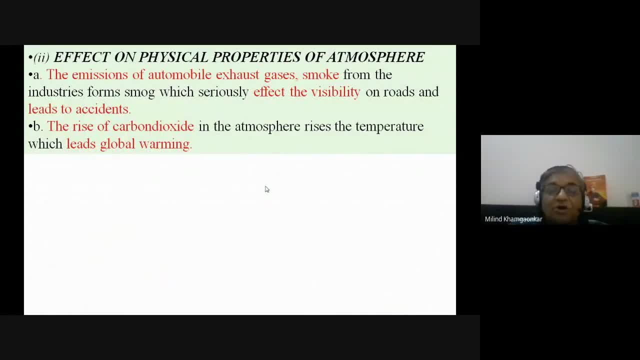 Now the next part. we have just seen the effect of this on the human health and the animal health, you can say. And the living birds will also have the same effect. Similarly, what will be the physical property of this in the atmosphere? 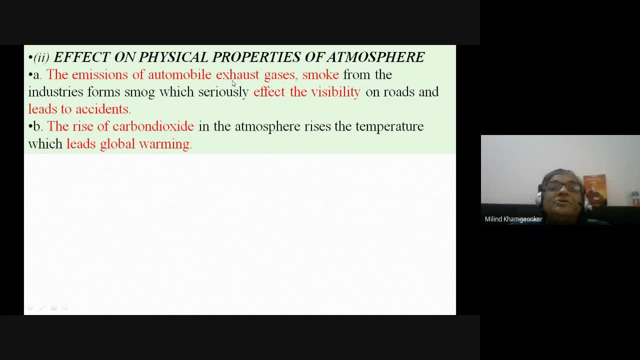 What will be the effect on this by the pollution. So the emission of the automobile exhaust gases or the smoke from the industries forms smog. That is again smoke and the fog together formed this smog. Smog means smoke and fog means very fine. 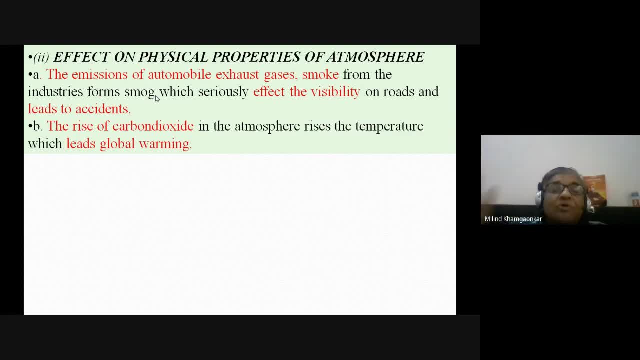 means not even vapour. we will call it water vapour, but not exactly vapour, but lesser temperature than the vapour, Mist, which is called smoke and the fog. that is the smog which seriously affects the visibility. If there is smog on the road, as I told you, if you go near Delhi, in Thandkale, then there is such smog. 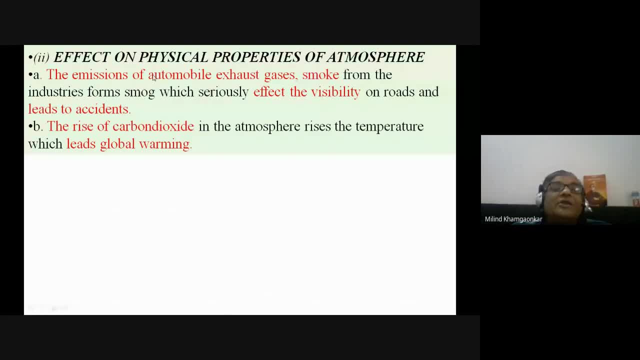 People burn the remaining garbage in the fields And due to the cold there is also fog, So both of them form smog and it comes on the roads. There are a lot of accidents there, So the effect of the visibility on the roads and leads to accident. 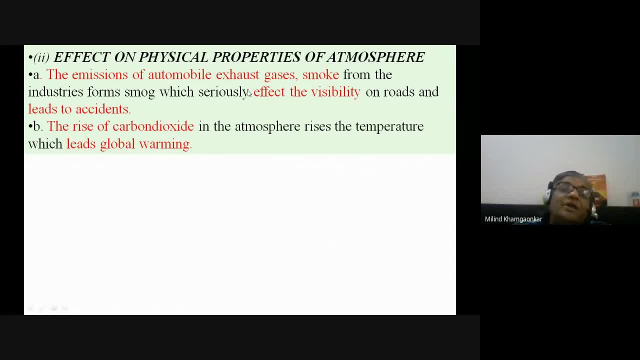 Also. that affects the aeroplane travel also, So at that time the air traffic in Delhi is also affected. The rise of this carbon dioxide in Delhi? Yes, Carbon dioxide in the atmosphere Rises. the temperature Leads to global warming. 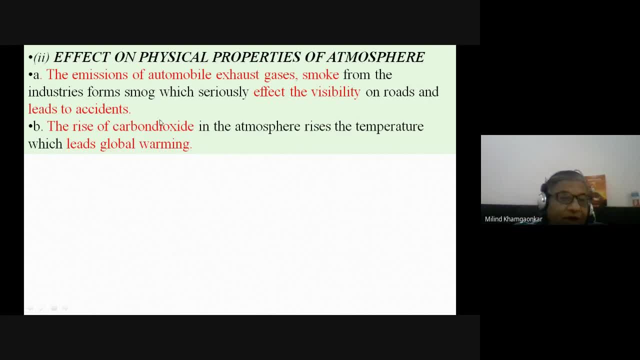 There is a greenhouse effect If carbon dioxide increases in the atmosphere because its weight remains very heavy, so it gets settled near the surface of the earth. It accumulates near the surface of the earth, And the bad property of this carbon dioxide is that it is a very bad conductor of the heat. 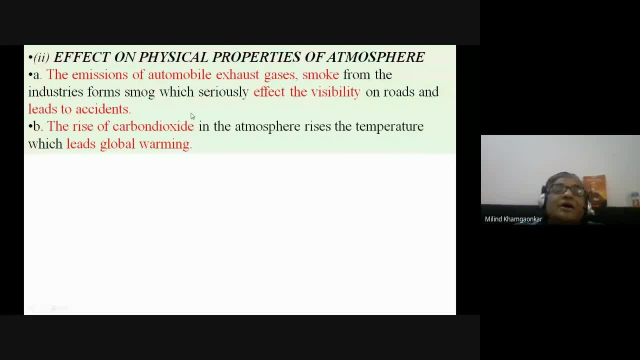 So the heat that comes from the atmosphere due to the sun does not let it reach the earth. It reflects the carbon dioxide. So the earth does not get the heat And whatever heat has come to the earth does not let it go out That carbon dioxide. 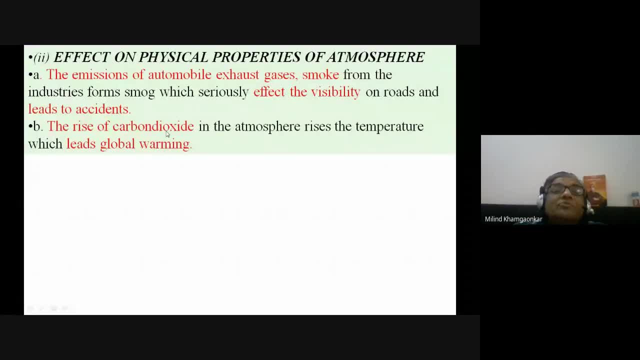 So the temperature of the earth keeps increasing. So both these things are called as the greenhouse effect. We make such a greenhouse Green, We make a house out of this green cloth And we like it inside. So what does that green cloth do? 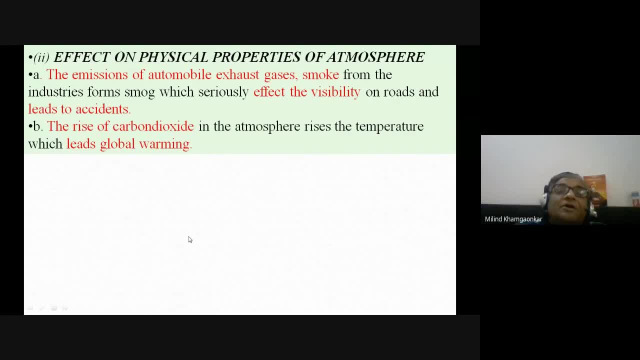 It does not let the outside sunlight come in And the humidity inside does not let it go out. So that is called as the greenhouse effect. That is being done by the carbon dioxide, So it increases the atmospheric temperature And ultimately, if the entire globe or earth is hot. 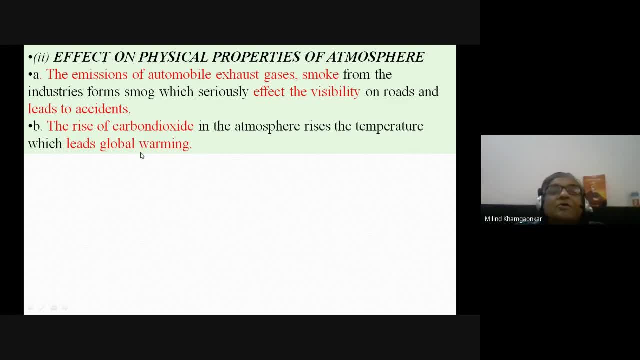 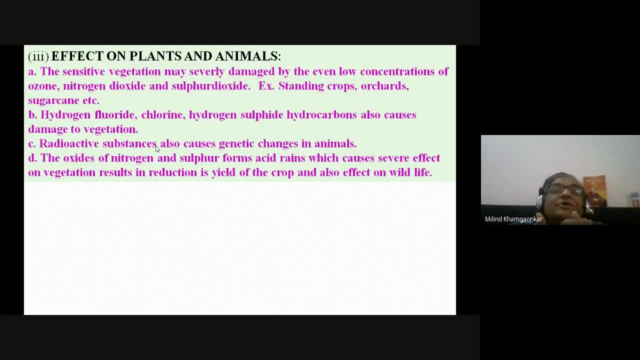 then it has global warming. Because of global warming, all the snow and ice melts. So in this way, how the properties on the earth are affected by the air pollution can be seen. Now the effect on the plants and animals, Naturally the sensitive vegetation. 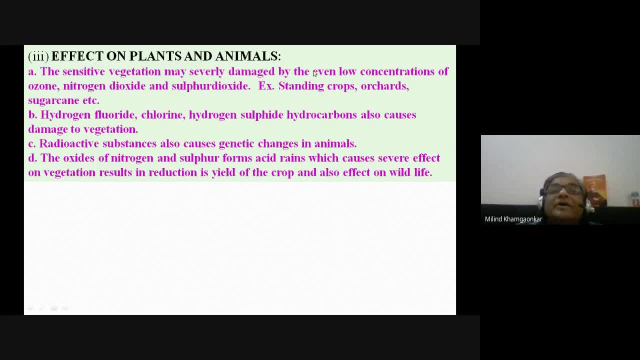 our crops, agricultural crops. they get damaged by low concentration of the ozone. nitrogen dioxide, sulfur dioxide, standing crops, orchards, sugarcane- they all get affected. Hydrogen, fluoride, chlorine, hydrogen sulfide hydrocarbon also causes damages to the vegetation. 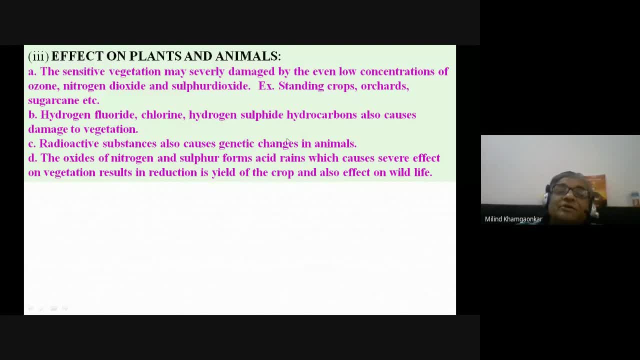 Radioactive substances also changes the genetic changes in the animals. In the animals their genes are the ones that change the radioactive pollution Right, If there are genetic changes, then in the next generation there will be faults and problems in them. There is cancer. 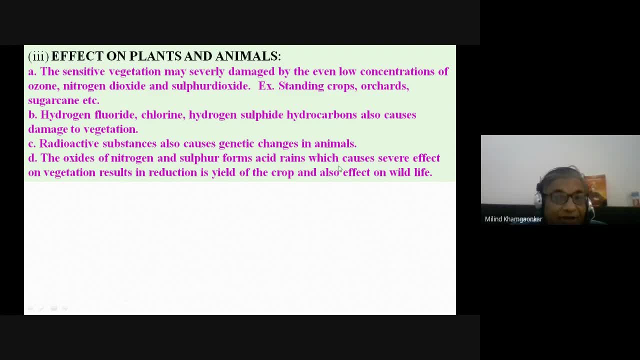 The oxides of the nitrogen and sulfur forms acid rain, which causes severe effect on vegetation, results in reduction in the yield of the crop and also affects the wildlife. You must have read about acid rain. It happens many times If there is a high amount of nitrogen or sulfur oxide in the atmosphere. 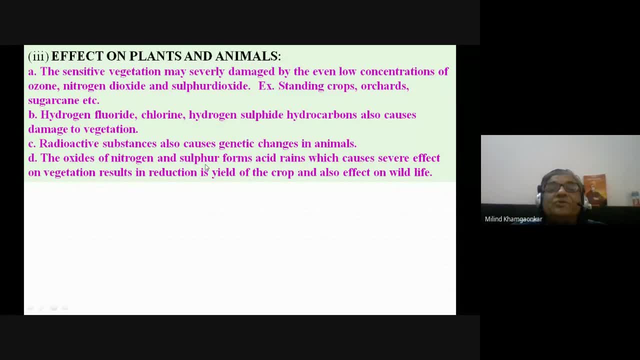 it mixes with water. it reacts with water to form H2SO4. And HNO3, nitric acid or the sulfuric acid. when it falls in the rainwater it damages the plants, the bushes the agriculture, It reduces its product. 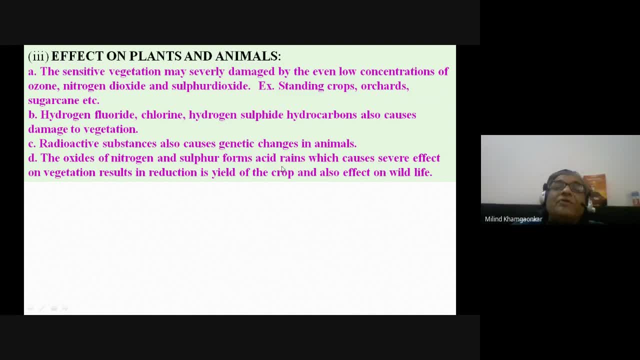 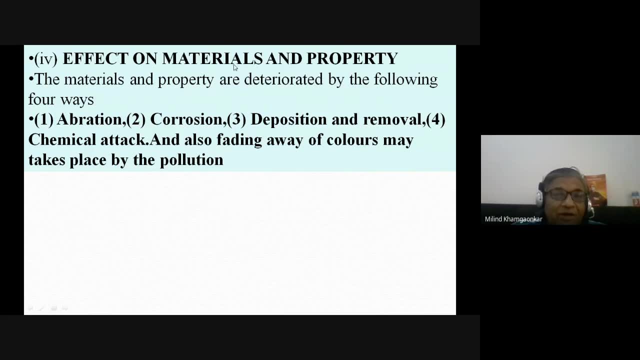 And it affects the wildlife or any animal that comes in that rain. Last is the effect on materials and property. Due to the air pollution, the materials and property are deteriorated by following four ways. I have told you the best example of this. 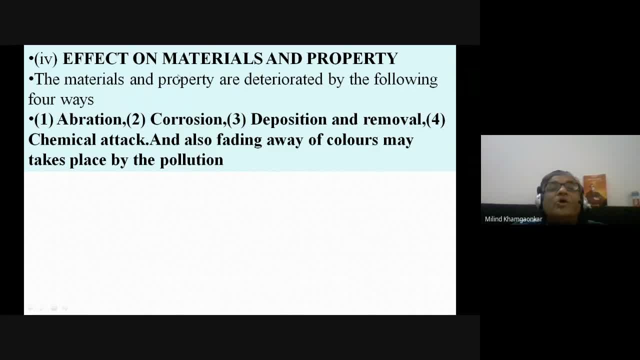 Taj Mahal. There are many such monumental buildings like this. There is Lal Quila Taj Mahal, there are some southern paita, there are temples on the side, there are many mountains, there are many ponds. All that they are getting damaged due to the air pollution. 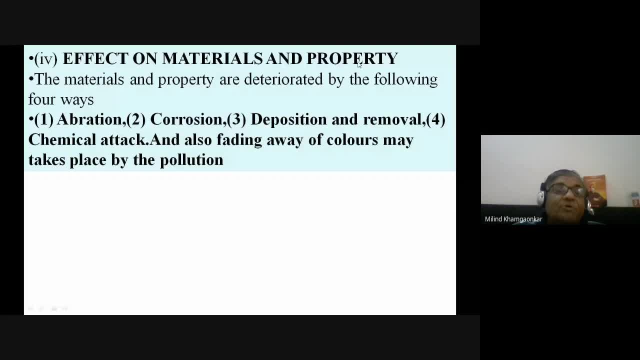 that comes under the materials and property. Why does it happen? What are the various phenomena that takes place due to the air pollution? They are the abrasion. Somewhere there is an abrasion in it, The surface, on the surface comes out. 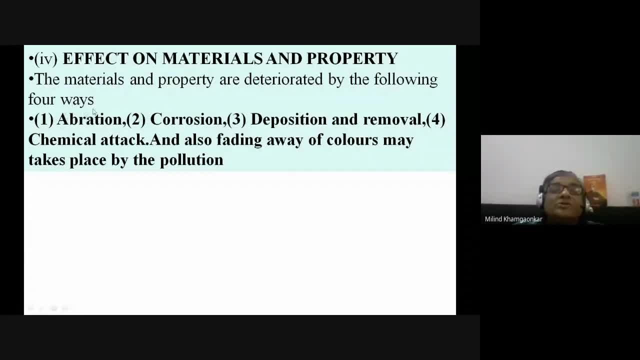 Abrasion, Corrosion, Sulfur dioxide, nitrogen oxide, chlorine. If they are present, excess in the atmosphere, they mix with water And the reinforcement in the concrete etc. gets corroded and results in the deterioration of the structure. 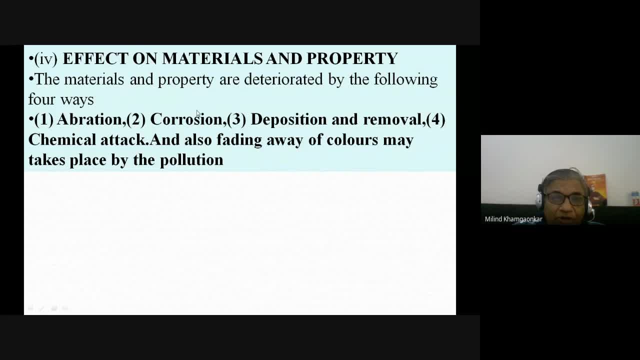 So that is the one of the cause of the air pollution. There is carbon dioxide in the air- CO2.. Nitrogen oxide is NO2.. Then there is sulfur dioxide, SO2.. There is chlorine- All these when mixes with the fog. 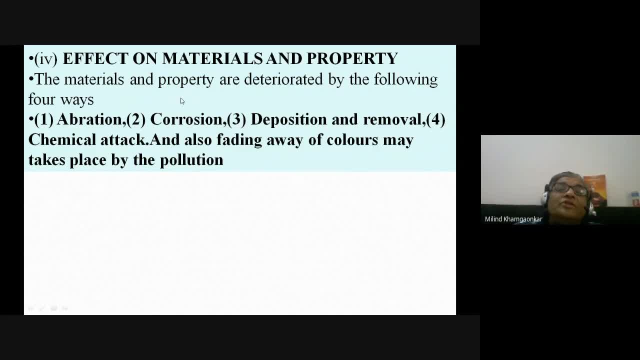 Or you can say smog, Smoke with the fog. So there results in formation of all those acids: Nitric acid, carbonic acid, sulfuric acid, hydrochlorides, HCl, chloric acid. So this results in the ultimate corrosion. 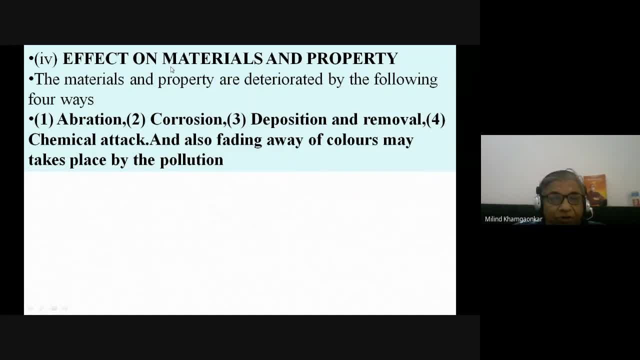 and destruction of the structures, Deposition and removal. Some chemicals are deposited Or the structure is deteriorated and removed. They also chemically attack. Also, fading away of the colours may take place by the pollution. The natural colour is due to pollution. 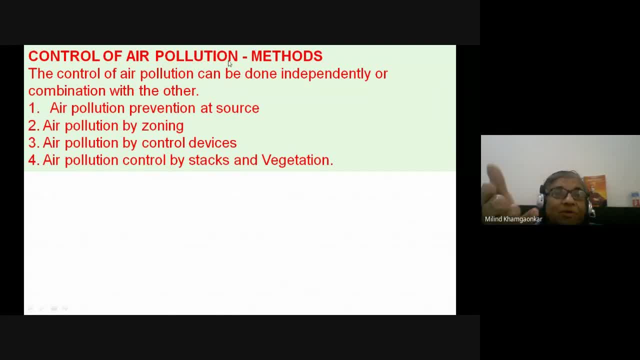 There are many examples of fading Like Taj Mahal is the best example. Earlier Taj Mahal was of white colour, So it started converting into the yellowish colour. Then studies were done on it. It was found that in Mathura, near the refinery, 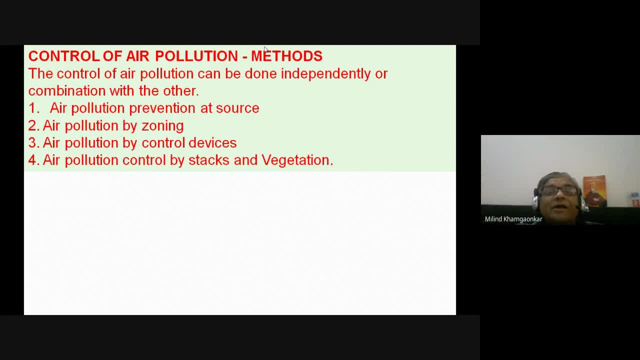 these gases come from there, And then they started doing certain protection work to the Taj Mahal Because it comes under the eight wonders of the world. The Taj Mahal is under the eight wonders of the world. Now, with this knowledge of the air pollution, 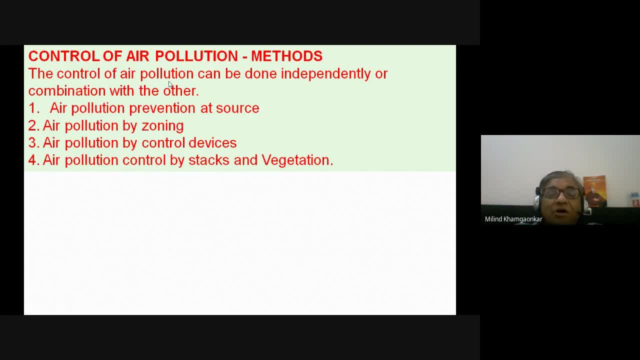 their sources, their causes, their effects. we will move on to the next and the last part of this air pollution, That is, the control of air pollution, Because now we know about our disease, We also know about its diagnosis. Now, what treatment do we have to give to it? 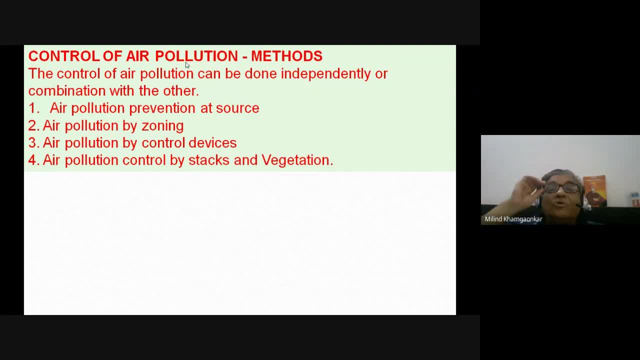 We don't have to leave it like this. The pollution will be a problem, But let us have certain measures or remedies to control the air pollution. So the control of air pollution can be done independently or combination with the other. Our air pollution at source. 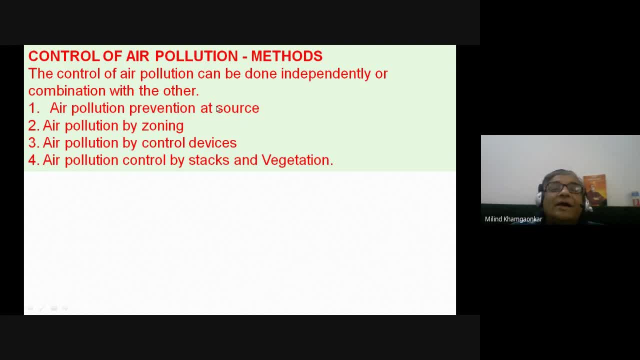 air pollution. prevention or control at source means from where air pollution is happening. arrange some such arrangement at the source itself that the air pollution is reduced. Improve in the machinery. your raw material should be of good quality Even after that, if there is air pollution. 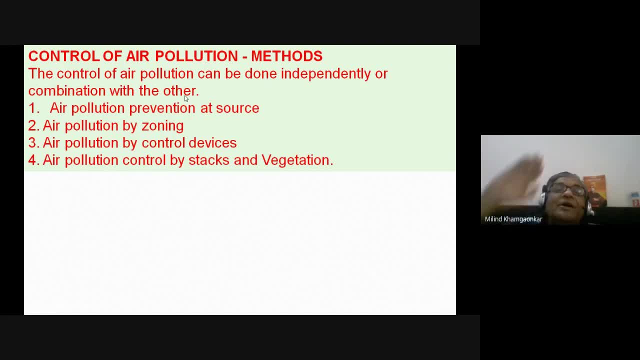 then somewhere, stack it or place a chimney and leave it in the atmosphere as much as possible. Leave it that much. Or, if there is any other gases that we can dissolve in water, that smoke can be passed through the water and it can be filtered. 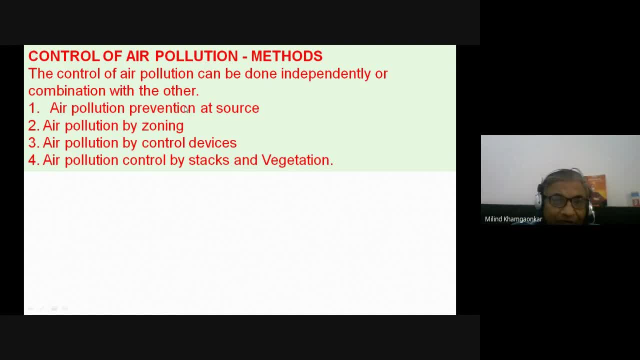 So all the various methods are there for the pollution control at the source That we will see. Then we will see the air pollution by zoning. What have we done now? All of you know that. what happened earlier, a long time ago, 40-50-60 years ago, 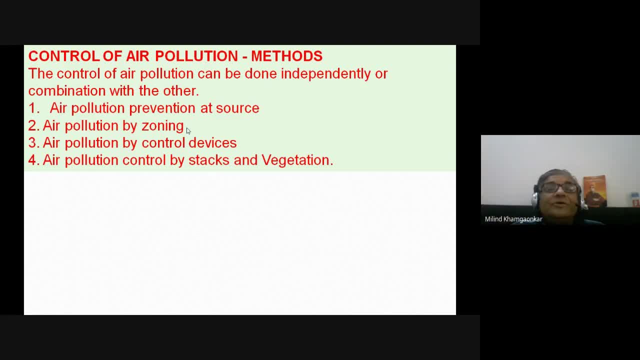 the industries were in the city. As you have seen even today that in some cities, like in Ahmedabad or in Surat or even in Bombay, all the industries which are producing pollution, they are located in the city. Some industries can be in our Nagpur as well. 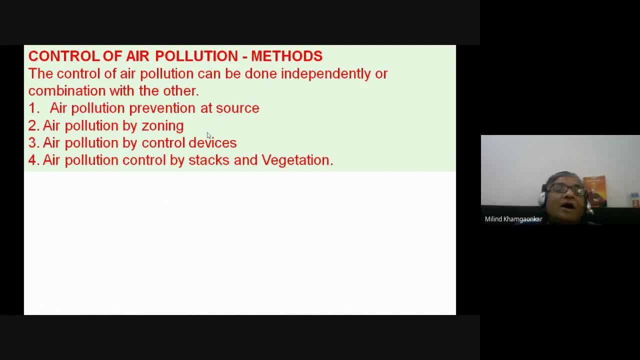 Like we went to the bus. stand there. you have Dalda industry. there is another industry. You can see that they are in the whole city. They are in our now, the one near Shukrawar Talaw. there was a cloth factory in olden times. 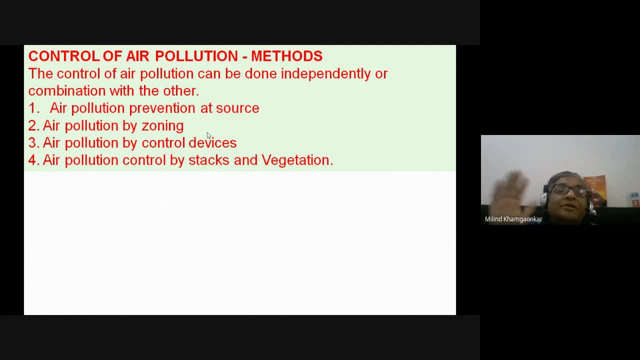 That too is closed now. but they were into the cities and producing pollution, air pollution into the city. So on top of that, then it was done that why not to concentrate the industry in certain zones, certain area to which we have given the name as 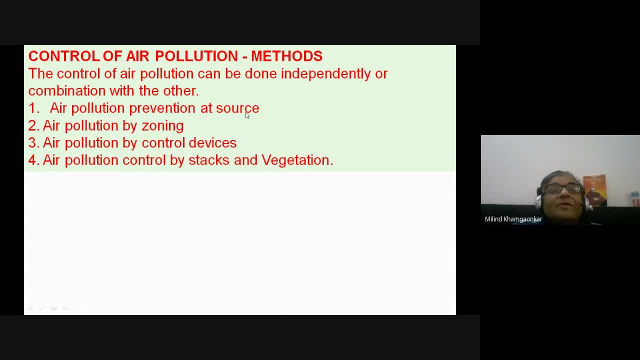 MIDC zone And Maharashtra Industrial Development Corporation's MIDC, like Butiburi MIDC somewhere. Hingana has MIDC somewhere. Wadi has MIDC, So outside the village or some other zone, even if there is pollution. 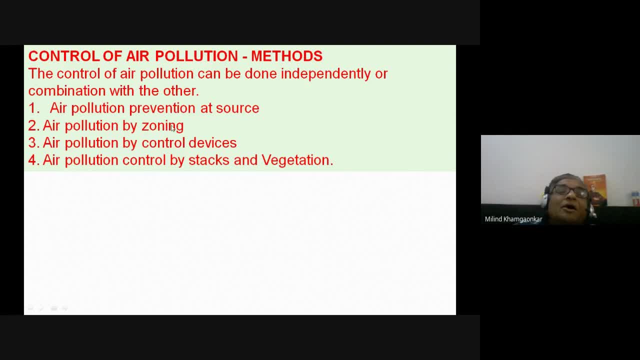 it will be there in one place, It will not be distributed, And then it will be tackled in that zone. So that is the air pollution by zoning. Air pollution control by certain control devices, some equipments, use of the equipments. 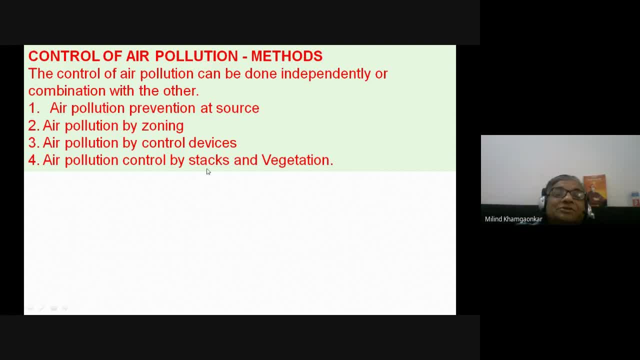 Air pollution control by stacks, Stacks and a chimney Or vegetation. If there is a forest, if there is a tree, if there is a bush, every plant is a source of oxygen. You all know, with the help of the photosynthesis, 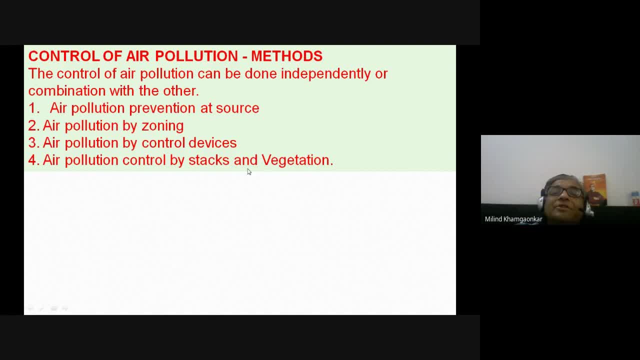 into its leaves, the leaves of the bushes. there is photosynthesis: Water from the soil, carbon dioxide, which is a greenhouse gas. that carbon dioxide from the atmosphere and the chlorophyll from the plant leaves together, the biological reaction takes place. 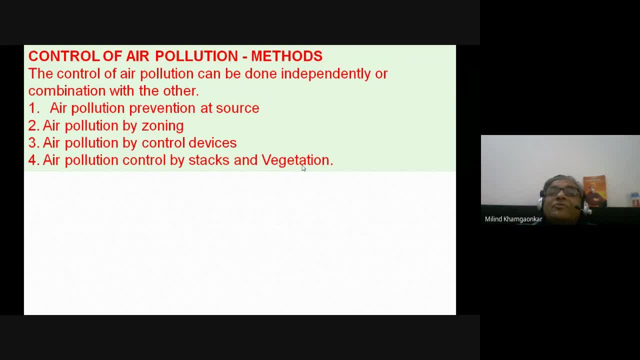 That is the photosynthesis And that converts that carbon dioxide into oxygen And some part of the water. So therefore, the vegetation is very important. It is very important to plant bushes. It is very easy to break it, But planting one bush. 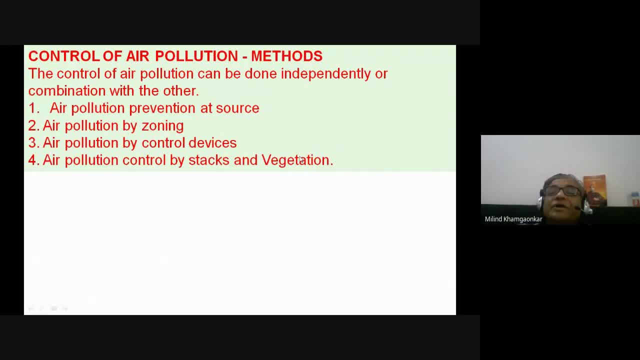 and growing it for 20-25 years is a very difficult task. If we see a ready-made bush, it has taken at least 25-30 years, But breaking it can be done in an hour. It is very easy to break. 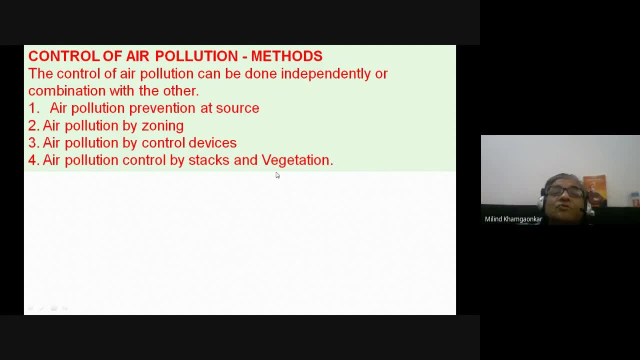 But it is very difficult to make, So vegetation is very important. Stacks, or what we call a chimney. look at This is the that you can say, pari, which is bringing all these air control measures. Okay, Now we will move on to the one by one. 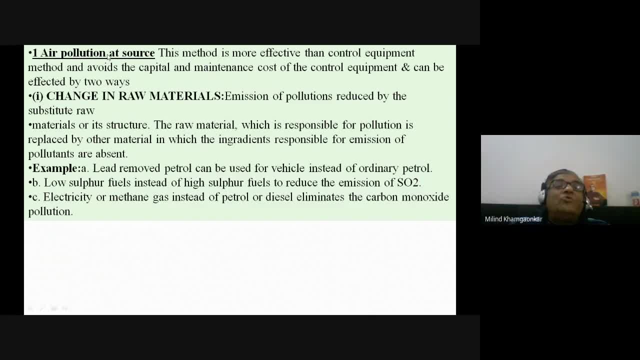 Air pollution at the source. How to control the air pollution at the source. This method is more effective than control equipment method and avoids the capital and maintenance cost of the control equipment and can be affected by two ways. That is from where the air pollution happens. 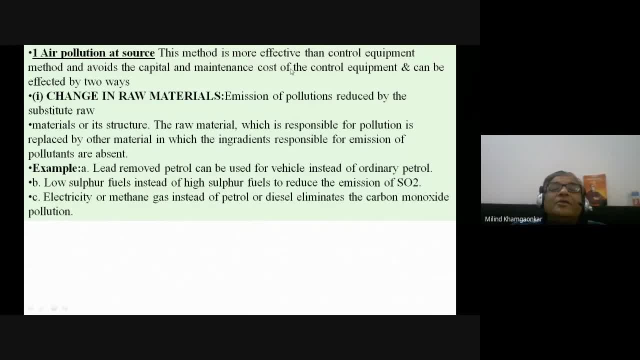 if we control it at the source, we can save money. Because of that, we have to use equipment, later spend and maintenance in the industry or in the machinery. that also can save money. What is that? Change in raw material. 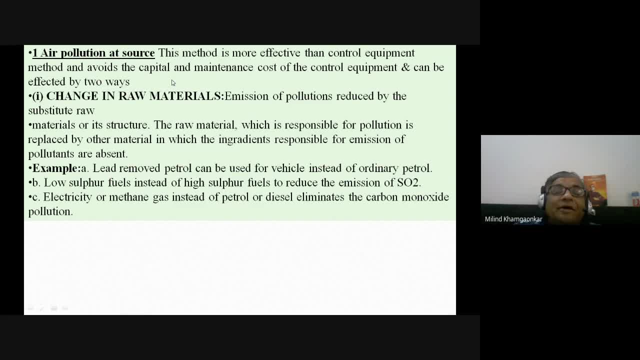 I told you that the raw material is a cement industry. In the cement industry, lime is used, calcium oxide and silt is used, or silica is used- SiO2.. So we get both of these from the mines. The mines are naturally occurring sources. 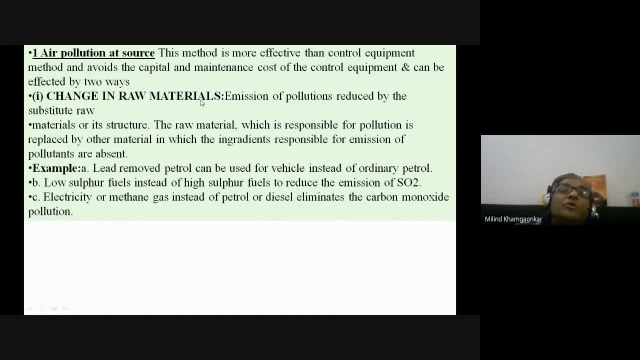 So there is a pure form in it and there is an impure form in it. In the coal industry, coal is found in the mines. In some mines the coal is pure and in some mines it is associated with the soil and the silt. 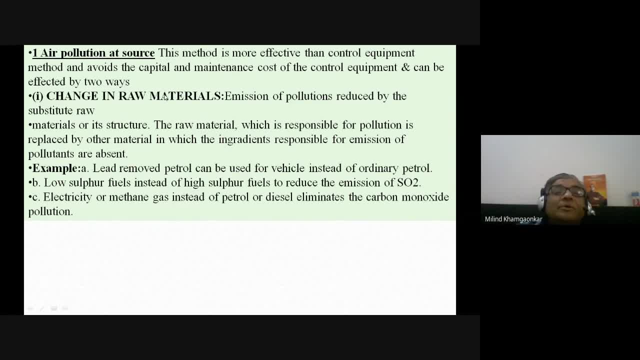 So what we have to do? We have to improve the quality of the raw material, either bringing it from the good quality mines or using the material by washing or cleaning it. So emission of the pollutants can be reduced by the substitute raw material or its structure. 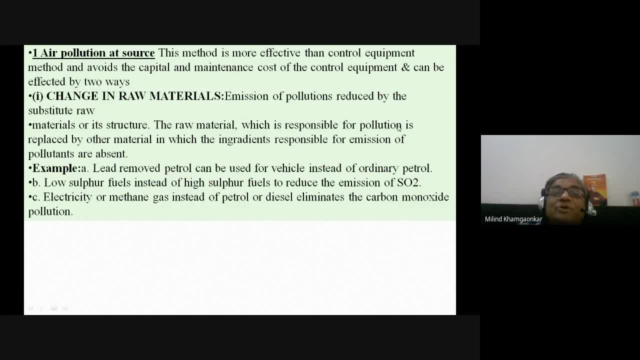 The raw material, which is responsible for pollution, is replaced by other material in which ingredients responsible for emission of pollutants are absent. For example, lead removed from petrol can be used for the vehicle instead of the ordinary petrol If we get the petrol from the refinery. 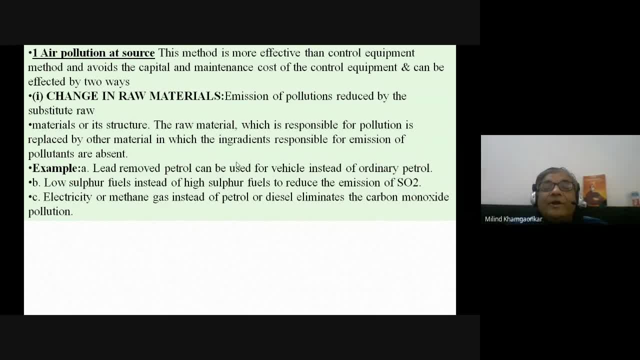 we get the oil from the mine. Petroleum from the mines or from the bowers can be used From there. we get the petrol oil, you can say, And it is then converted into petrol, diesel, rock oil, etc. into the refinery. 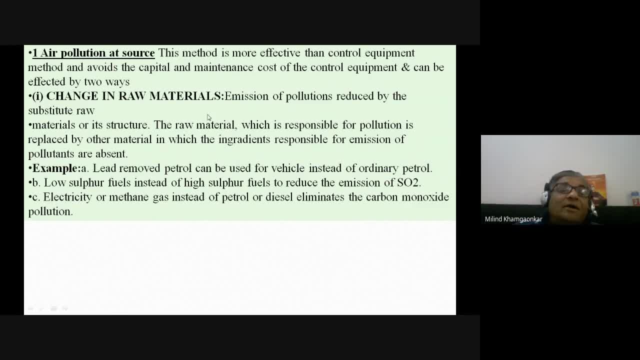 But in that petrol, while converting the lead, Pb is being getting added and that lead is injurious to the machinery that creates the lead oil. It creates the lead oxide, oxygen, lead oxide into the emission of the vehicles And that lead oxide, PbO2. 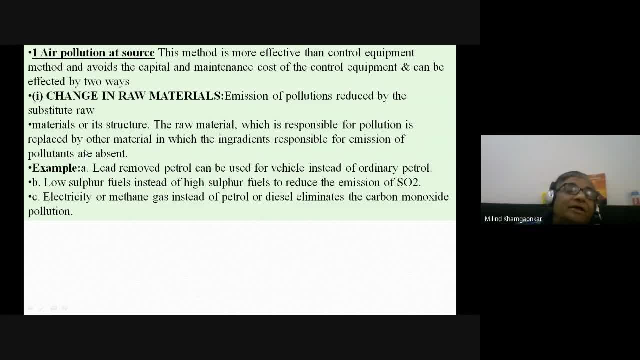 is very dangerous for the human. If we extract that lead from the petrol, then that is the example of the raw material improvisation or the air pollution control at source. The petrol we get now from the petrol pump that is without lead, we get the petrol. 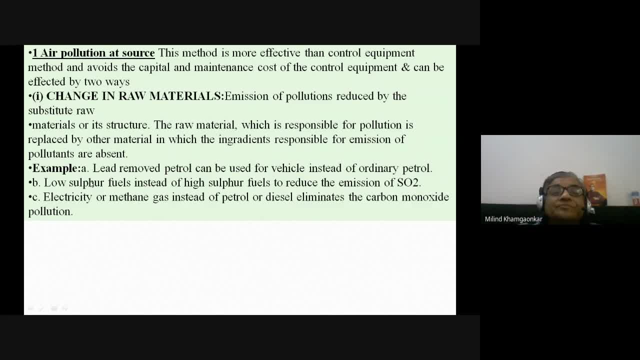 So that is one of the examples. Second example is low sulphur fuels instead of high sulphur fuels to reduce the emission of the sulphur dioxide, SO2.. The fuel we have- petrol, diesel- should have at least a little bit of sulphur. 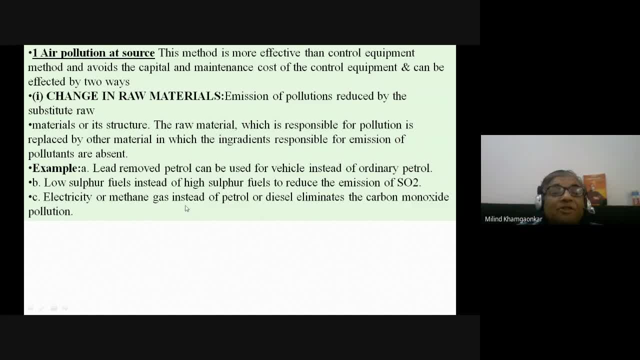 Electricity or the methane gas instead of the petrol or diesel, eliminate the carbon monoxide pollution. You all know that Nowadays the automobile industry is moving from use of the petrol or diesel First. it has moved to the LPG, liquid petroleum gas. 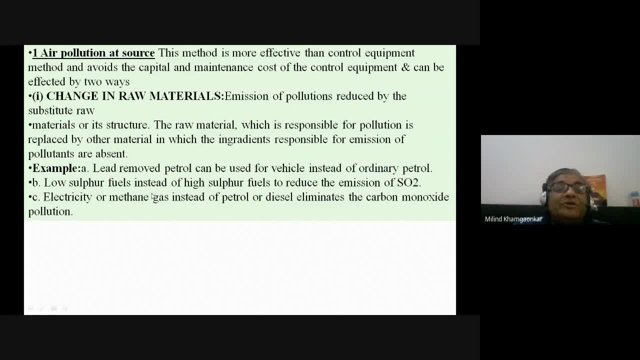 or liquid nitrogen gas, LNG. Now vehicles are running on methane gas. Some cars two-wheeler, four-wheeler or the three-wheelers, And nowadays, the next generation vehicles are coming. They are the electrical vehicles. They run on electricity. 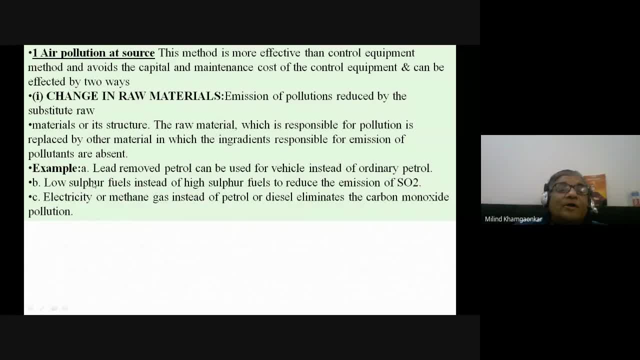 on the batteries. So no production of the carbon monoxide or carbon dioxide. So this is one of the examples of the air pollution control at the source. So very good. three examples: Lead removed from petrol, Sulphur removed from the fuels. 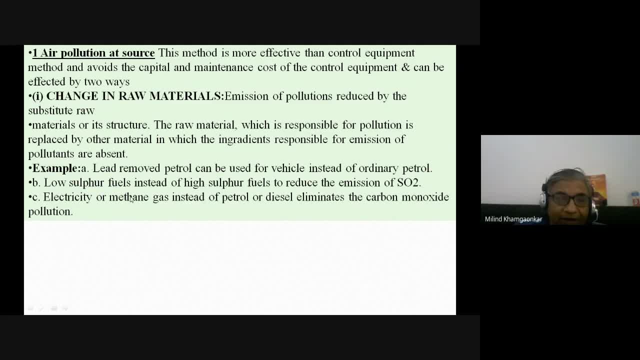 Or lowering the sulphur quantity And electricity, or methane or LPG or LNG is called liquid petroleum gas or liquid nitrogen natural gas, LNG. In Nagpur, in many places there are gas pumps And from there the gas is being given. 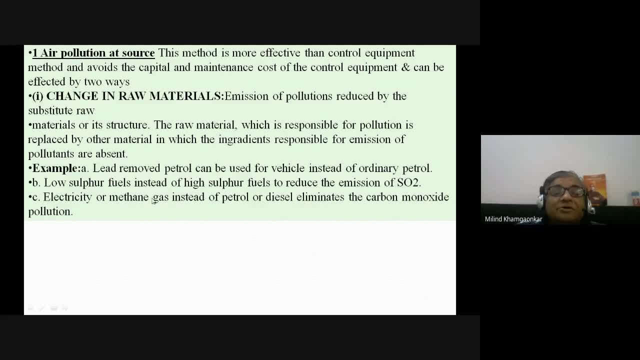 like the petrol, like the diesel. So these gas, these engines which work on these gases, they work more efficiently, Lesser carbon dioxide and carbon monoxide is produced And they give more average. Also, now the electrical vehicles have come. 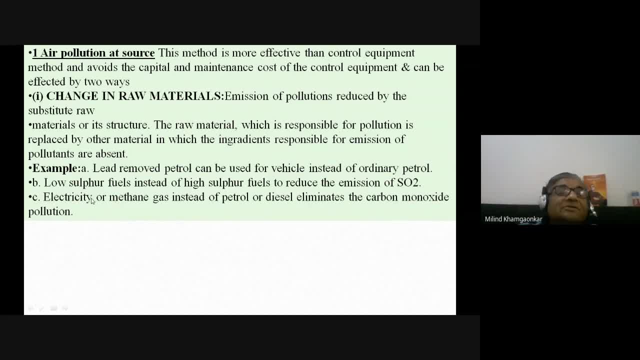 You must have seen. various cars are there. Various three-wheelers are there, Various two-wheelers are there, And the cars which run on electricity, the four-wheeler. which colour number plate does it have? Tell me tomorrow. I have given you. 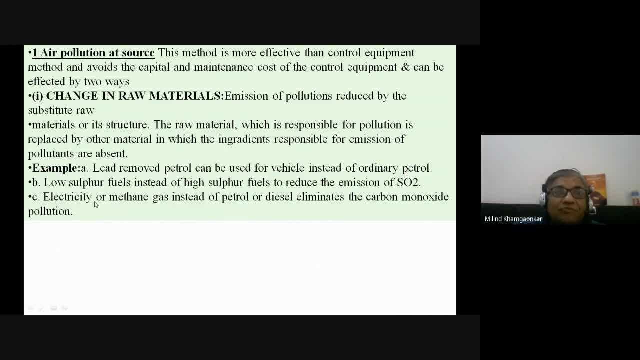 two questions today: The vehicles which run on electricity. it has got different colour name plate, number plate. So if you think so, you can tell me tomorrow Or you can tell me at the end of the lecture. There is no problem. 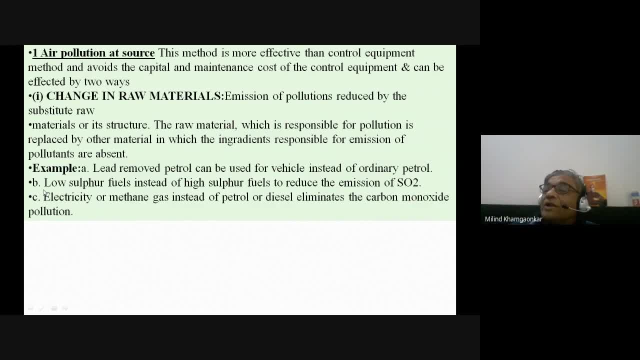 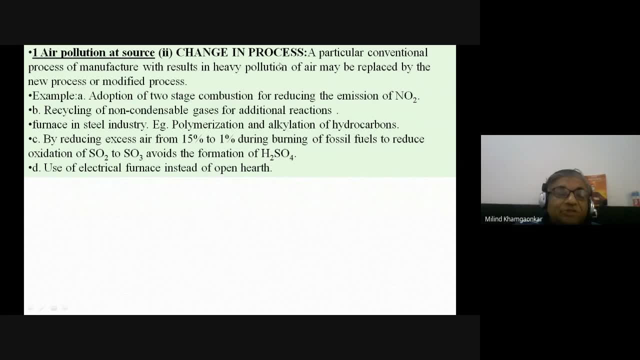 You can tell me in the last part of our lecture. Now we will move on to the next part of our discussion, That is, the change of the process or the second method to control the air pollution, A particular conventional process of manufacture which result. 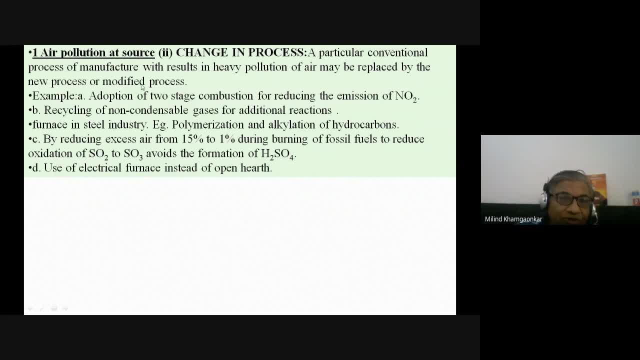 in heavy pollution of air may be replaced by the new process or modified process, The industry of old times or the old machines. the equipment of old times means not older generation, but the you can say older machineries can be replaced. 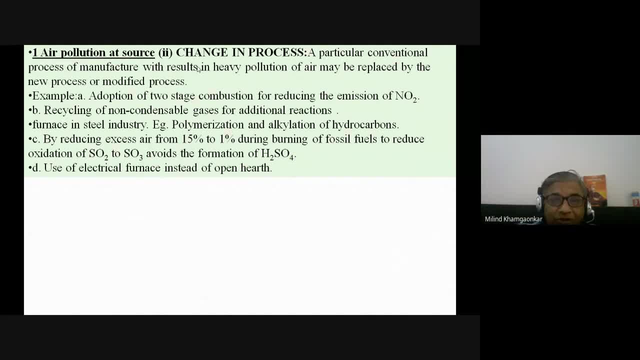 with the new technological machineries. Nowadays there are new machines, new electronic technologies, So there is less manual interference and less pollution production. So it should be done like that. So in that means the equipment should be refined. 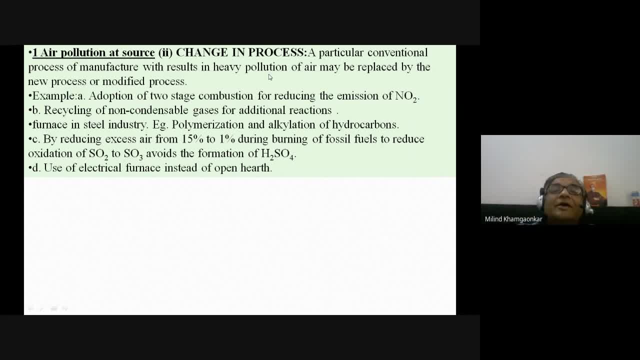 Now there is a cloth industry. There are new equipment in that, So we should have a cloth machinery. Cement production industry has changed a lot So we can reduce the pollution in cement production. There is a lot of change in the thermal power plant. 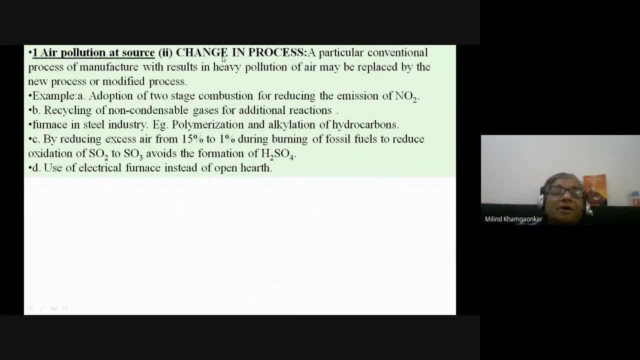 too. So everywhere there are advancement or automation in the industry. So with the help of that we can change the process of the production and then we can improve the process and we can reduce the pollution. the various examples are given: adoption of the two-stage combustion for reducing the 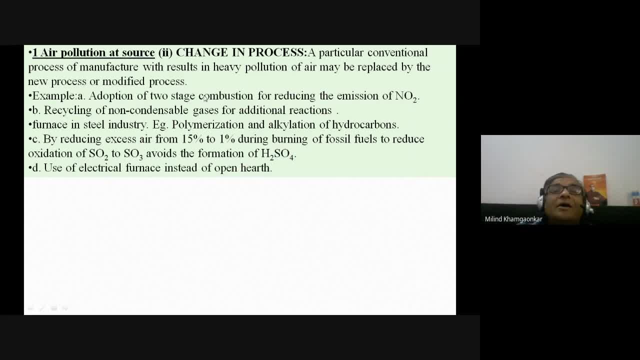 emission of the nitrogen oxide. and our a one stroke engine was there. then there were two stroke engines, cycle. what happens in those engines? all the fuel, maximum part of the fuel, is converted into energy cycle or car or aeroplane engine electrical energy. you can say so during that combustion conversion, the combustion of the 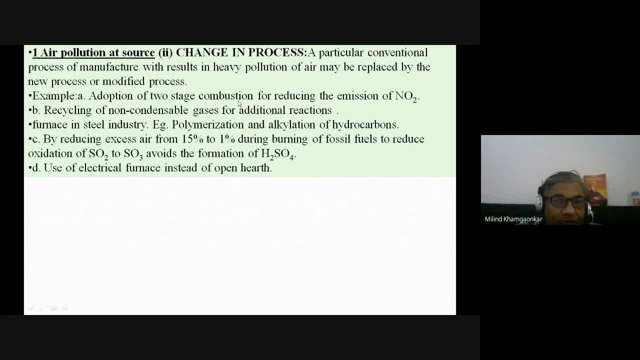 fuel should be hundred percent, no pollution. but due to certain flaws into the engines, yeah, non-advancement, or the fume you can say. so two, one stage, one stroke, two strokes, a little four stroke. okay, i have a maybe which amari job, four wheelers. 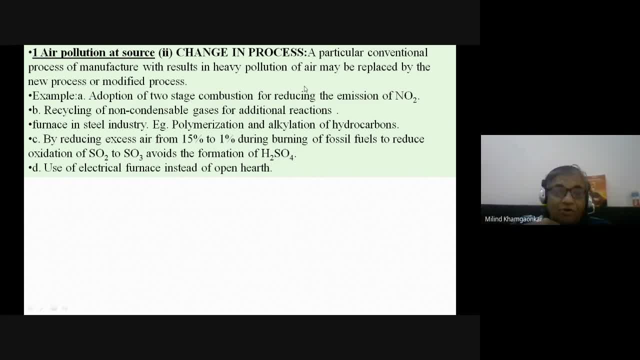 a this may, or advanced engines- okay, my knowledge is up to only four stroke now. the recycling of the non-condensable gases for additional reactions and a? a gases produce hotel academy industry. message your polluted gases. say so usko, recycle kernel, usko reuse kernel a. 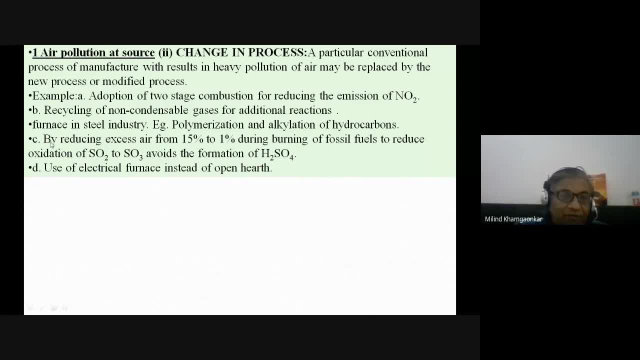 b, a change in process, mega furnace in steel industry. steel industry, me jo, but yeah i boiler. i furnace a usme improvisation: polymerization and alkylation of the hydrocarbons, then by reducing excess air from fifteen percent to one percent during burning of the fossil fuels to reduce the oxidation of so2 to so3. 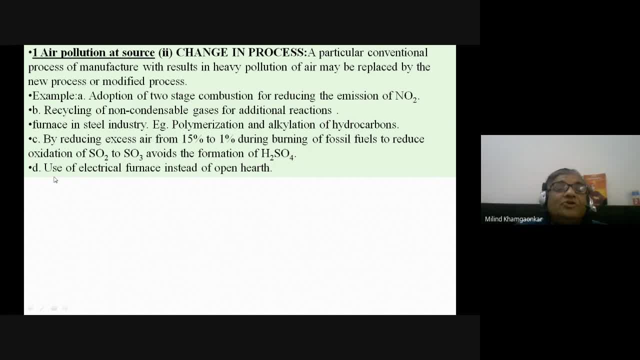 avoids formation of the h2so4. use of the electrical furnace instead of the open heart. we think this is as g. i fire gas if u dispers at brее and an electrical gas is酒 furnaces are also there. we in Nagpur we have all the three. that is electrical. 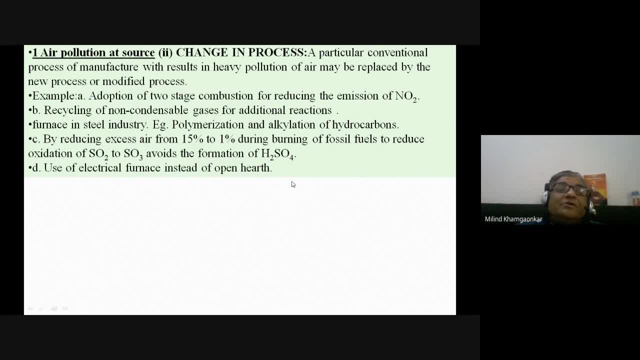 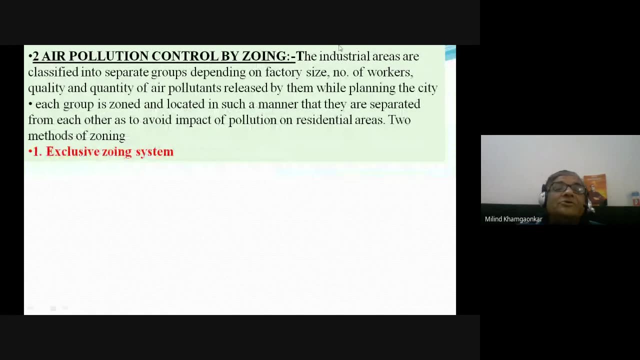 furnace, gas furnace and the by the natural resources- wood, etc. so this is again the change in the process to control the pollution. now we will move on to the last part and we will continue our discussion in our Leslie next lecture regarding the air pollution control by zoning and a man, a copa data. 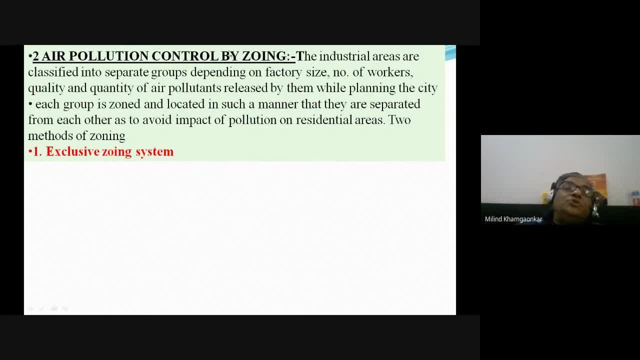 key in the olden days. as you will move to I'm the bath, you will move to surat, you will move to bomb a Mumbai, to Pune or any big cities, or maybe in certain small cities like the Incan, God, etc. wherein all those industries are. 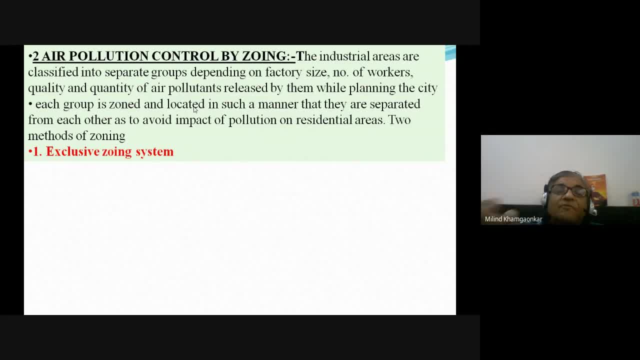 located in the olden days, as you will move to Ahmedabad, you will move to Surat in the Olden days as you will move to Surat. the iron factories, the tineries, that is, the leather industry, all are located inside the city and that the industry is located in the inside the city are now. 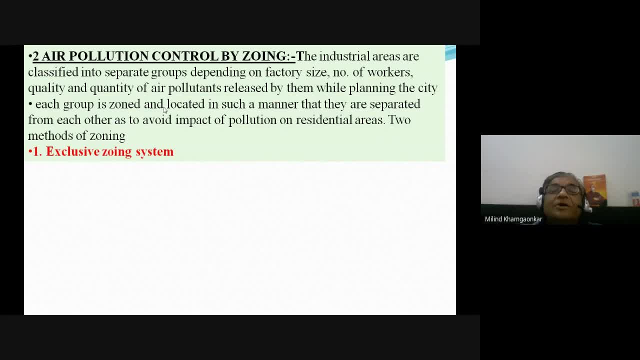 hammering or hampering to the people living nearby by the air pollution. so now, therefore, that it has been decided to zone, to locate these industries into the certain specific area to which we called as the MIDC area Maharashtra industrial development corporation for Maharashtra, Bihar, make a BIDC yoga Bihar industrial development corporation, or came at the 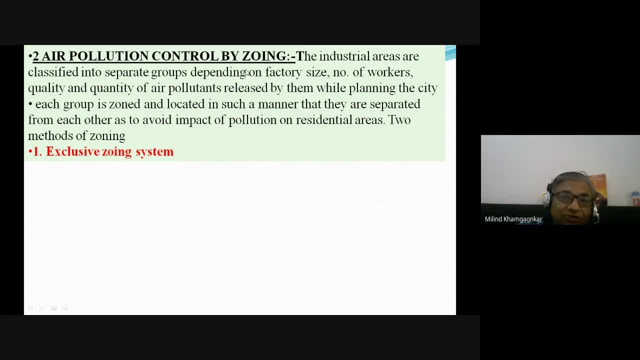 Pradesh with a medium at the Pradesh yoga. so that is the zoning, that is the locating the industries in certain zones. like we in our Nakpur, we have booty Buri, five-star MIDC, the Hingana MIDC, the Wadi MIDC, and every city has got the. 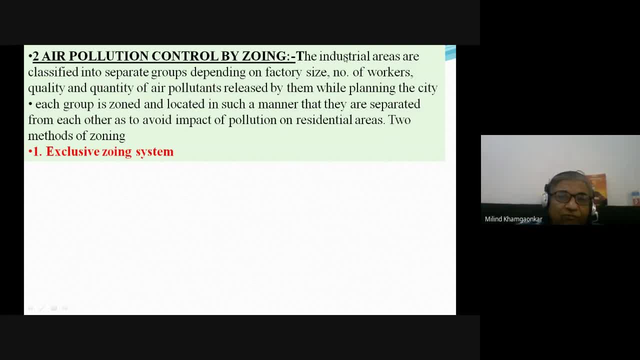 MIDC. other benefits are also there for the industries, so the industrial areas are classified into the separate groups depending on the factory size, number of the workers, quality and quantity of the air pollutants released by them. while planning the city city coplan car, they work. he is watching it. each group is 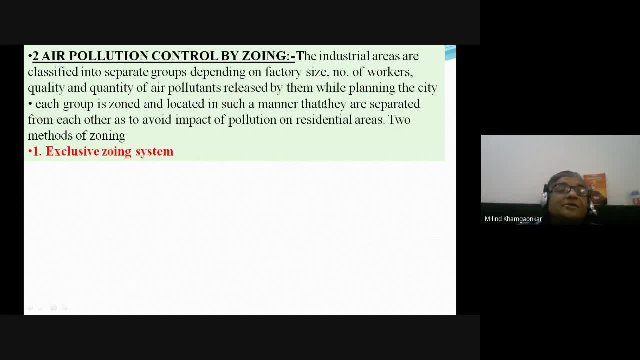 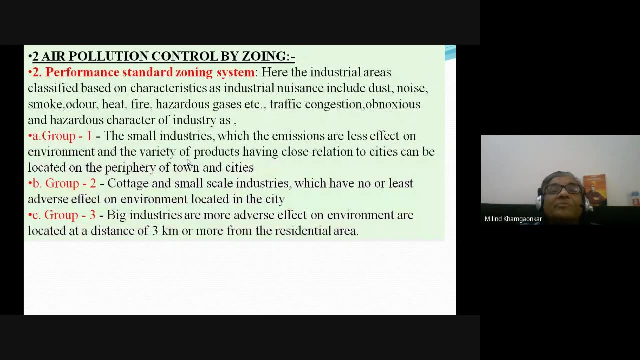 zoned and located in such a manner that they are separated from each other as to avoid the impact of pollution on the residential areas. two methods of the zoning, that is, the exclusive zoning system and the performance standard zoning system. these we will discuss in our next lecture. we will take the break. 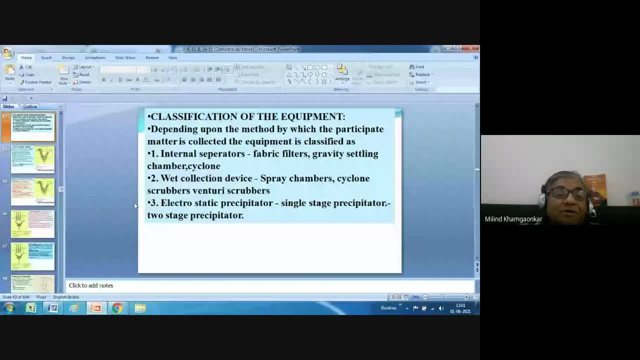 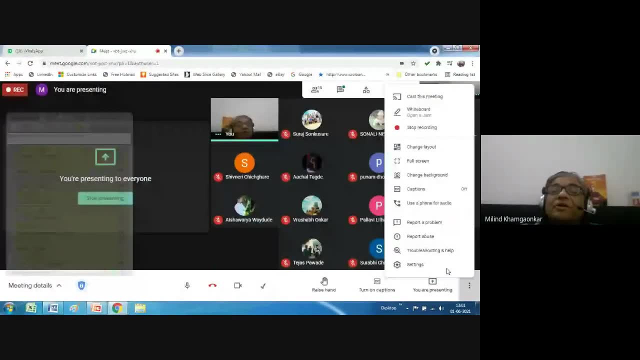 here another, the equipments, etc. in our next two lectures we will try to